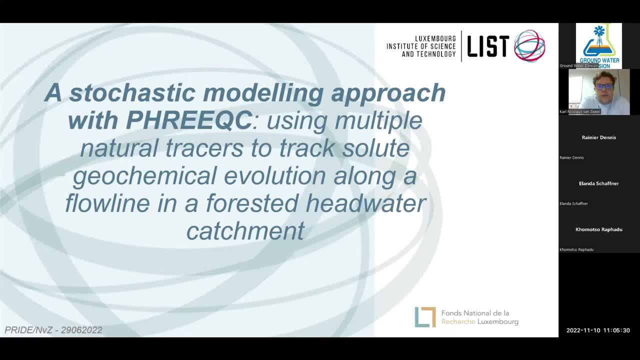 the title of the talk today is the Stochastic Modelling Approach of Frick C, Using Multiple Natural Trace Tests to Track Solid Geochemical Evolution Along a Flow Line in a Porositeal, And I'm going to give you a bit of background. So just to give a bit of background. I'm moved away a bit from mining. 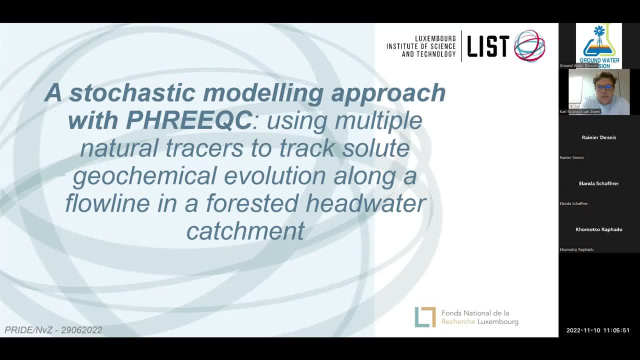 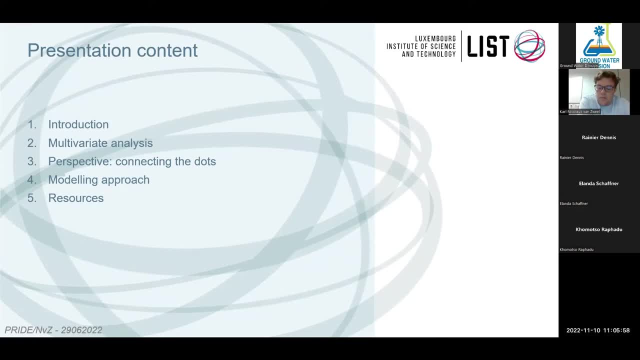 geochemistry and I'm working now more in chemistry. So the PhD is sort of a bridge between hydrology as it is practiced in Europe. It's a bit different than what you probably are used to in South Africa. It's much more focused on travel times. 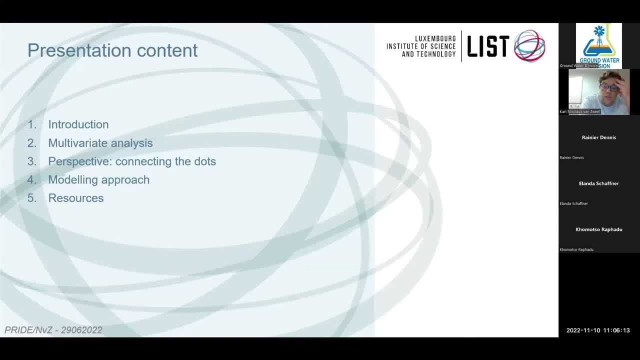 It's a big field in terms of trying to predict floods, so really into the stable isotope geochemistry and so on. But my side is a bit more looking at geogenic solutes, so calcium and magnesium stuff that might be used as traces that are coming from weathering of slates, especially in our catchment. 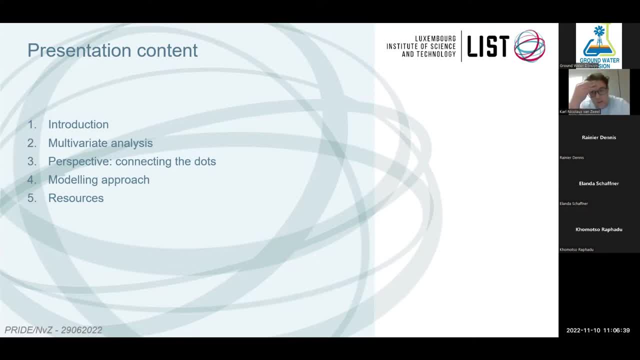 So our presentation will go. we'll give a brief introduction about my topic and the data we work with. Then I will go a bit into the multivariate analysis. We did a substantial amount of statistical analysis and a bit of machine learning techniques to sort of untangle the whole. 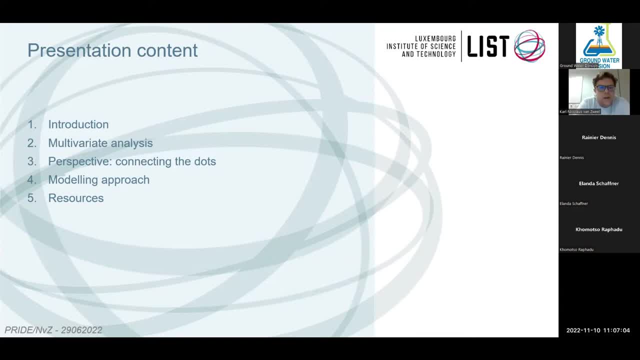 process, or all the processes that might be taking place, And then I'll just show how the model is working And then I'll move over to what we did In terms of what we did in terms of the industry as such, the industry as such. 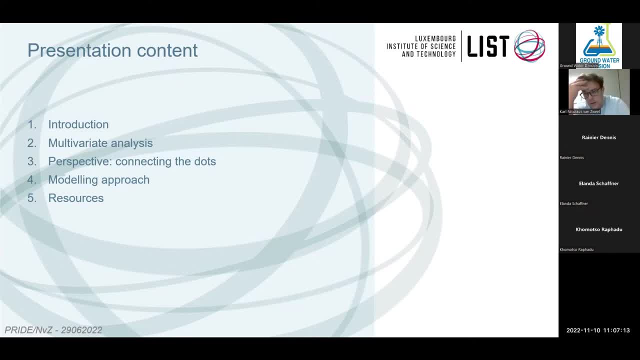 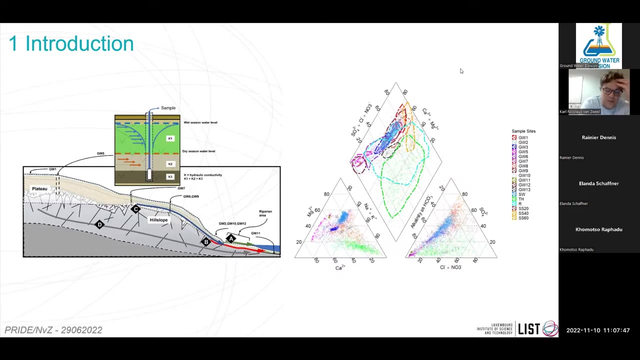 of geochemical modeling to see if the behaviors that we observe through the multivariate analysis is an actual fact, things that's happening, or so you know. catch that. so it's not in the sandstones, it's a dominion slate. so my I'm not a geologist. I might mispronouncing some of this stuff. I. 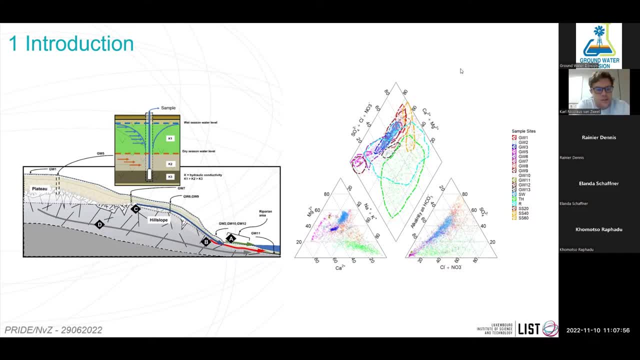 apologize for that, but the basic things are. it's just slates. but what makes this catchment really interesting is that the soils are not autogenic, meaning that they were deposited there via glacier movement and so on. so in normal weathering models you would expect that the soils would form. 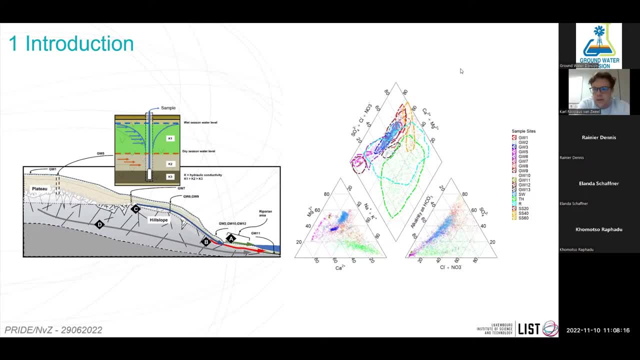 from the bedrock and that they will be depleted in with that material. but this is in our case not what is happening. we still have some primary minerals in the soil, so you have weathering in the bedrock. so your sort of weathering front that is moving down is in various stages of 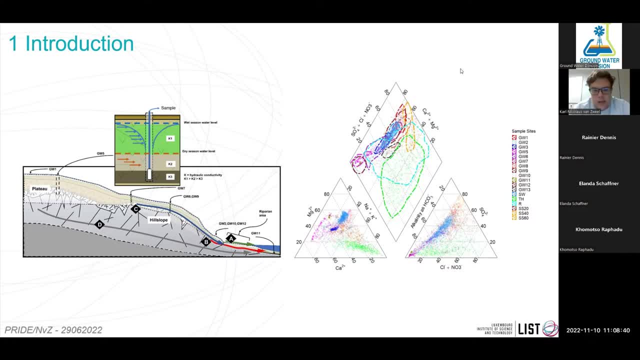 of weathering, so in terms of what is happening in flow generation. so the whole process, or the whole PhD project, is centered around trying to figure out how to predict the sort of the discharge chemistry, so meaning the little stream in the catchment, and a lot of isotope work has been done. 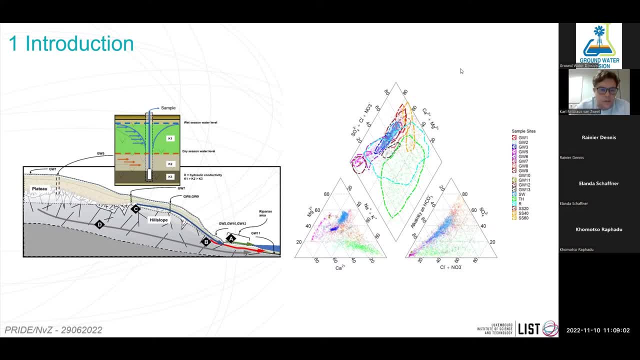 and they are fairly confident with the type of flow lines that you can observe in terms of stream flow generation, because we have what is often seen in a water catchment is a double peak flood response. so in terms of rainfall, you have an initial hydrograph peak and then it subsides. 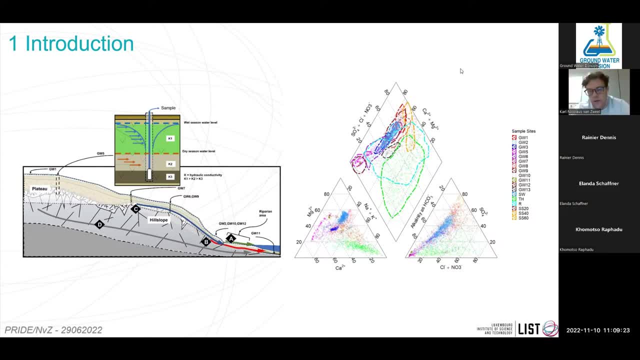 and then the secondary peak or a much larger and continuous peak arrives. so it is a mobilization of newer waters that is stored in the catchment. so to sort of just simplify it in the schematic, what you can see here is a transect of the hill slope and then you have a highly fractured 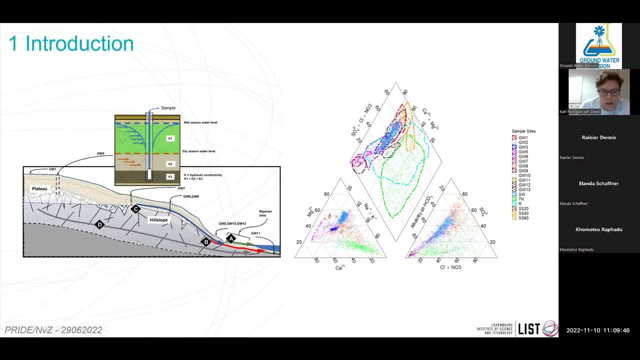 slade bedrock, and the flow line that moves through that is flow line d. and then you have this sort of weathered- really weathered, where you still have pieces of rock and soil and so on, mineralized soil mixture. so there you have a flow line called 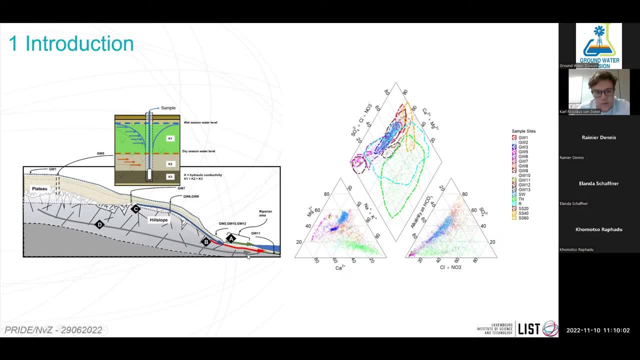 B. this is the one that is in close proximity to the stream And as the system weds up and you get sort of the saturation wedge that forms up the slope, you start getting a flow line C. So this is a mixture of what is rapidly infiltrating through the highly porous soils. 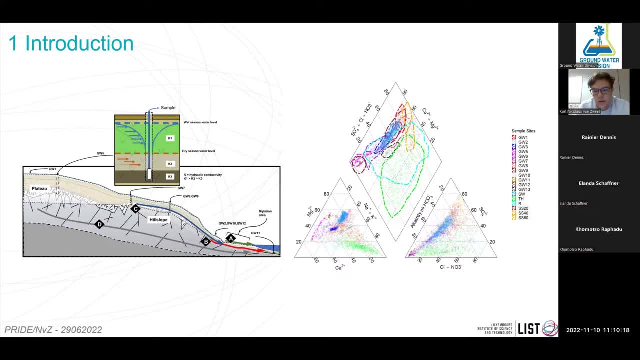 and then mixing on this sort of contact between the weathered and unweathered zone, And then it flows to the stream And then we have quite some substantial influences of the riparian zone around the stream. So this also alters the chemistry. So, in terms of the data set, the list has been monitoring this experimental catchment for nearly 10 years. 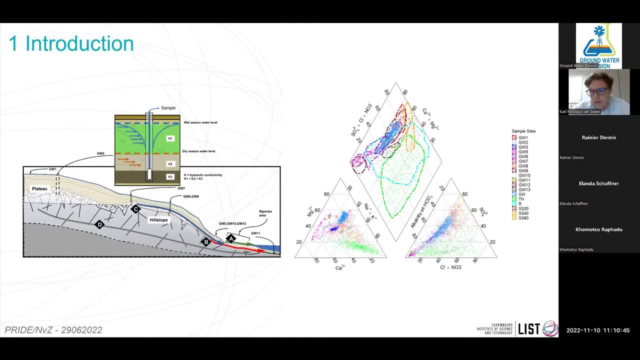 So we have biweekly chemical analysis of around 13 wells, But now the monitoring grid has been extended to 27 wells And just to give you an idea of the magnitude of monitoring, the catchment is only 14,. no, I apologize, 42 hectares, really small. 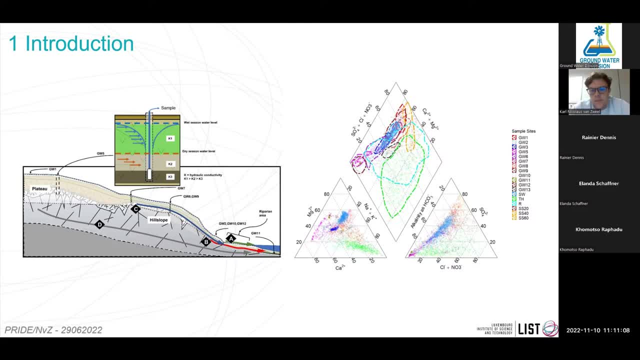 So we have a lot of wells And basically all of the wells that I studied are on a transect of the stream, So I could really track the flow of water as it recharges on the plateau and on the slope, And our data. 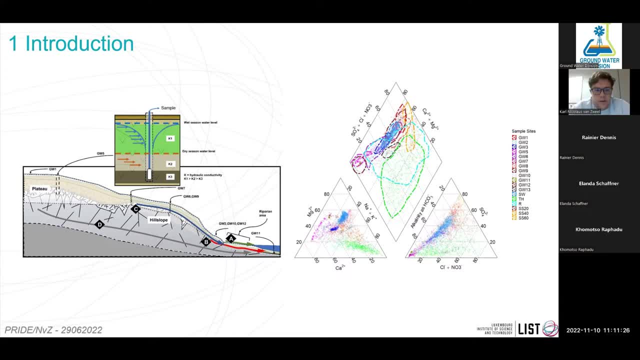 So I have about 6,000, 5,800 odd observations with 40 parameters. So it's major cations and anions and also ICT data and a lot of soil solution data as well. So if we look at the Piper diagram you can already see there's some interesting trends. 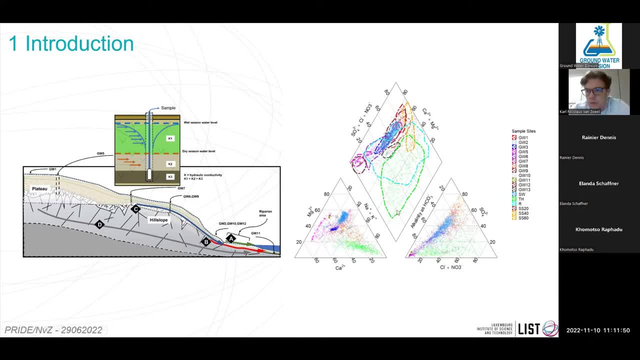 So this sort of light green color is a throughfall because the catchment is covered by, you know, by a mixture of vegetation, So spruce and Douglas fir. So this vegetation has an influence on what is input in terms of chemistry, but also we monitored dust deposition and obviously the pure rainfall as well. 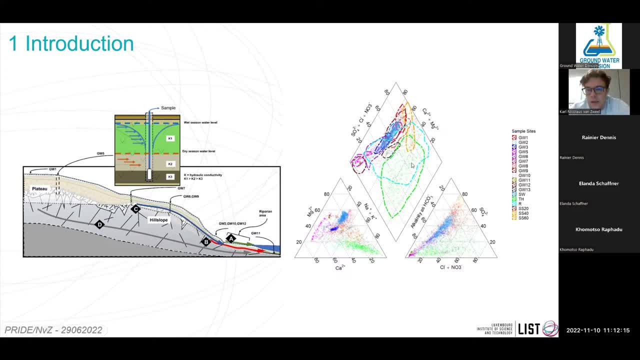 So the pure rainfall is the blue cluster, And then this sort of light brown color is the soil water composition, And the clusters that you see here are all groundwater clusters, Right, so already you can see there's sort of a trend, So you move from the freshly recharged water through the soil. 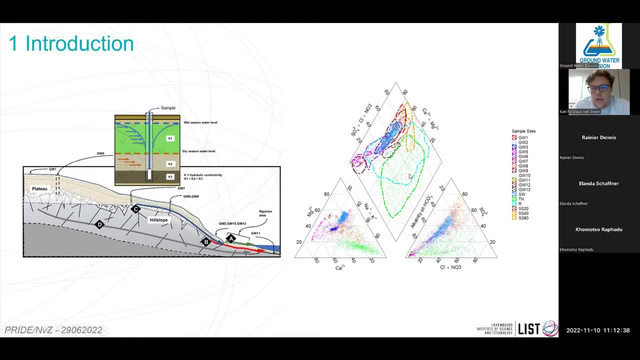 So it moves from a potassium sodium chloride dominated zone. It goes to more of a calcium, magnesium, sulfate type water, And as it moves to the deeper part of the water, the relative contribution of sulfate decreases and the relative contribution of alkalinity increases. 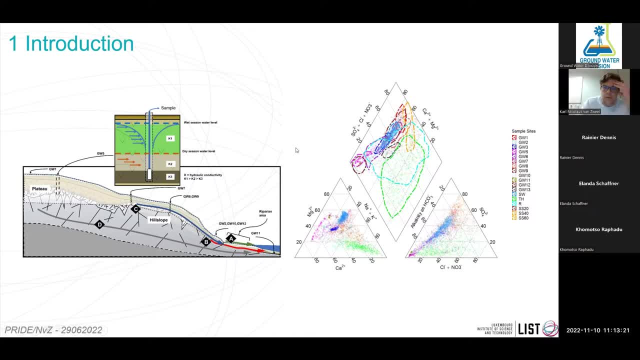 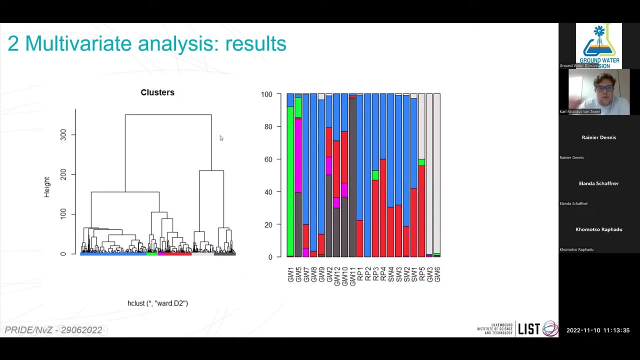 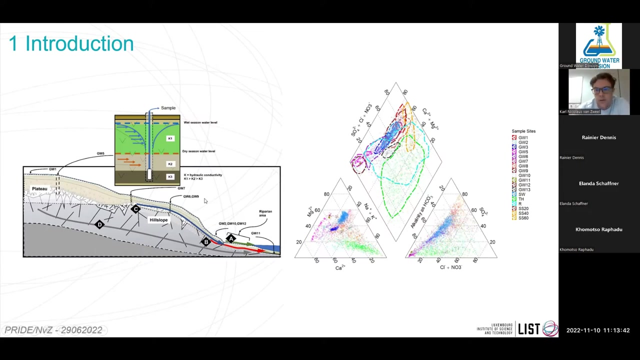 So this would have been the initial guess of what is happening. in terms of chemistry, It's sort of just the titration, where you have acidic soil water and it gets buffeted by some base. So then what we did is because- just to quickly go back- the problem is our wells intercept various flow lines. 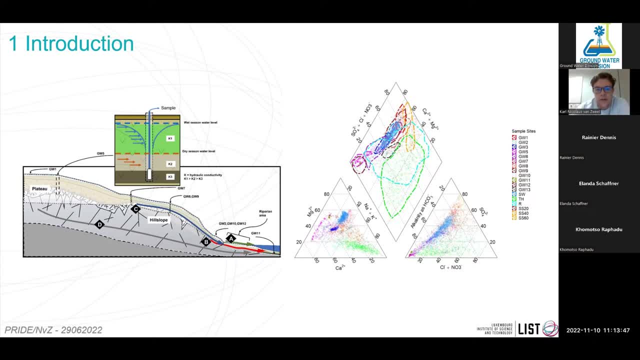 And because you have a really high variance in terms Of vertical conductivity due to the soil being deposited there and it's not weathered, you have- if the system is wet, you have- really high lateral conductivity And as it dries out, obviously the conductivity decreases. 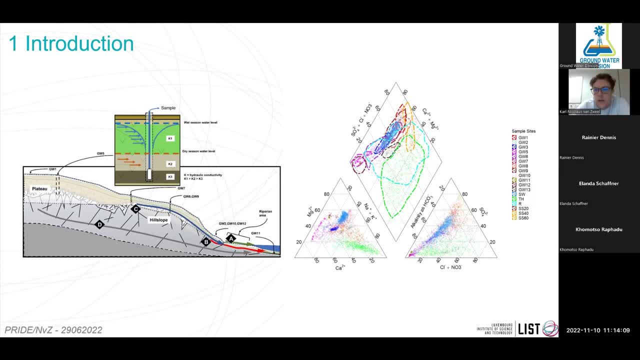 So if you were to sample in a wet season, you're more or less will only be drawing in water from the shallow flow lines, And as you, obviously the system dries out a bit- you start Getting the contributions from deeper flow lines, or you can see the signal at least. 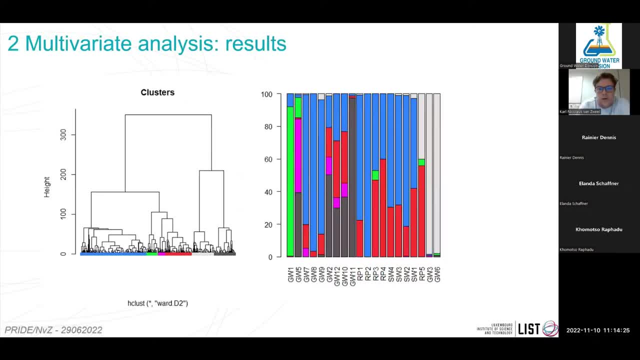 So what we did is we just do- is a simple our archaeological clustering. So you can see that the endogram on the left hand side, and initially we we cut the tree at around six main clusters And we just did an assessment to see the frequency of occurrence of these clusters in our various wells that we were monitoring and see if it makes sense. And we just did an assessment to see the frequency of occurrence of these clusters in our various wells that we were monitoring and see if it makes sense. And we just did an assessment to see the frequency of occurrence of these clusters in our various wells that we were monitoring and see if it makes sense. 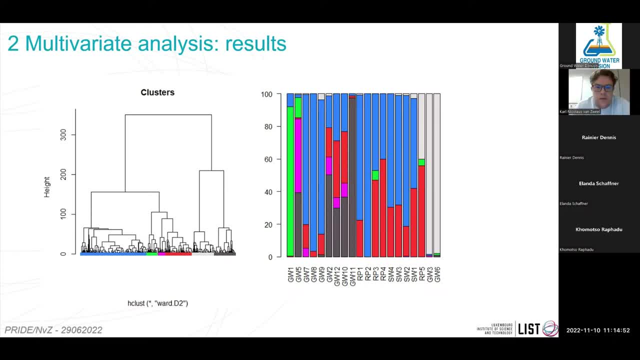 Okay And so, and this is what I want to highlight to myself- And indeed it's really predicted it quite well. So this blue is more or less what is observed in the stream, but you can see it in most of the shallow wells, meaning that what we expected, that most of the stream flow, is coming from this. 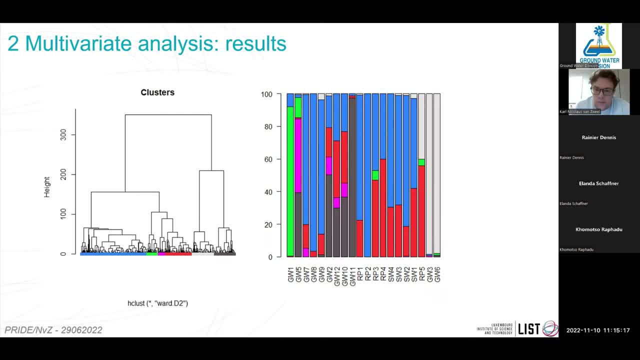 Shallower sections of our catchment, and this is what we wanted to do is to go a bit more in-depth to see if we can sort of explain the clusters, and we moved the phenomenon one step down, so cutting the tree to 13 clusters. so what i'll? 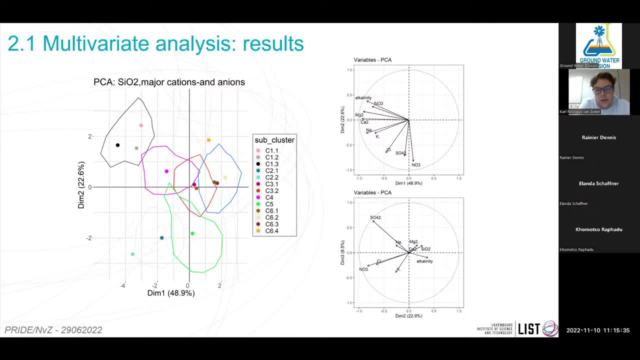 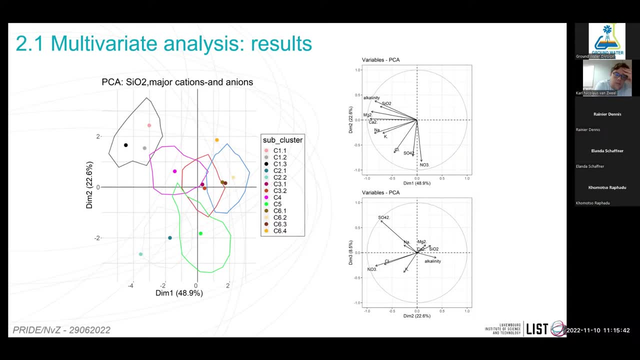 show you then, is we classified the samples or just labeled them, and that we, then we did a principal component analysis. so principal component analysis is a multivariate statistical analysis. we aim to just explain the variance in the data in terms of loading vectors, so to see what, how, the parameters, 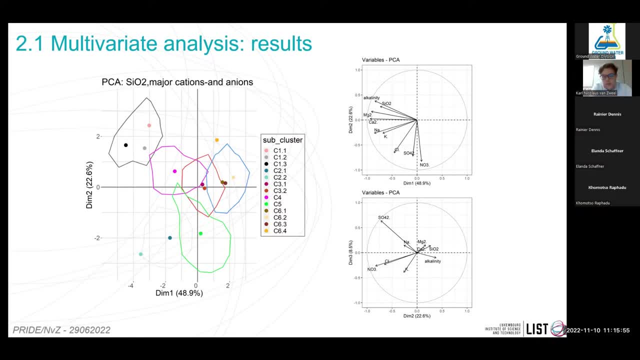 that we measure can explain the variance that we see in the data or why the clusters are are separating, right. so this polygons that you see here is the initial big classes of six classes that we made. so the dark one is the sort of deeper water that we observed and this purple cluster. 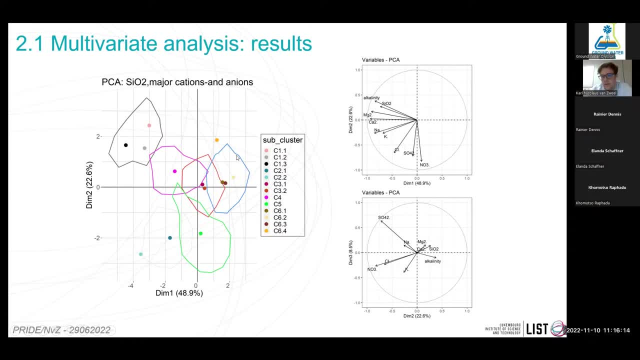 i'll get to in a minute. and then this red cluster and the blue cluster is the two um, the two sort of uh, um chemistries we observe in the stream. so the red is, uh, the red cluster is base flow, so when it is dry, and the blue cluster is when it is completely wet, so, um, and then uh, 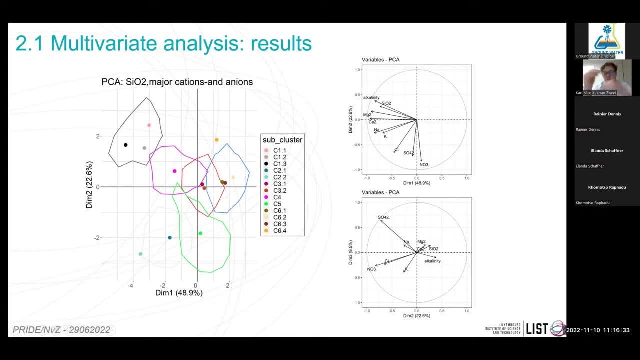 this green cluster is uh on the plateau. so just to quickly give you uh, just a bit of background, our, our catchment has two uh plateau or two heel slopes. so the one is what we refer to as the primary yield slope, so this is the the largest part of the catchment, but then we have a smaller secondary. 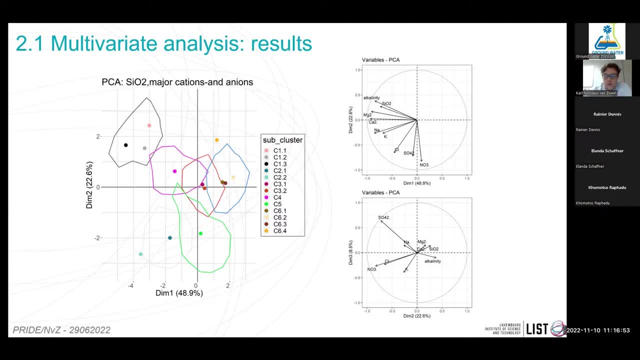 hill slope and the secondary yield slope, the soil layer on top of it. it's uh homogeneous. but on the primary plateau we have quite a significant weathering front. but what is interesting is that this weathering front has a cutoff in terms of elevation. so the base of the of the weathering front you can observe on the. 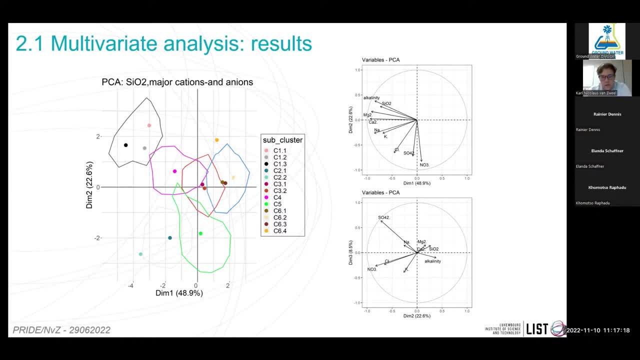 slope. so below this on the yield slope, you have unweathered drop. so this interplay between this weathered zone, where you have a bit more high conductivity, and chemistry- the chemistry also is a bit different- and how these units interact with each other in terms of 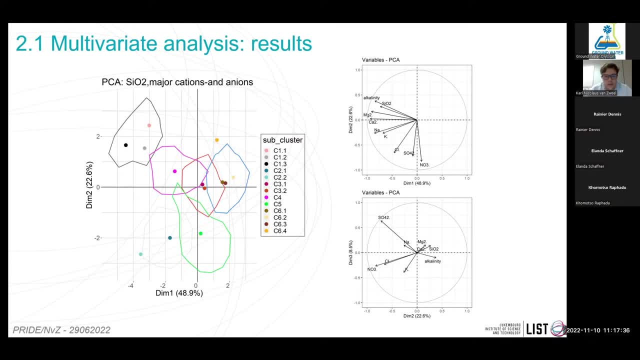 hydrological status and really what this phd is about. but i will not go into too much detail about that because i can keep you- uh- here the whole day and i think it's not super interesting for most. um, but i will not go into too much detail about that because i can keep you here the whole day and it is not super interesting for most. 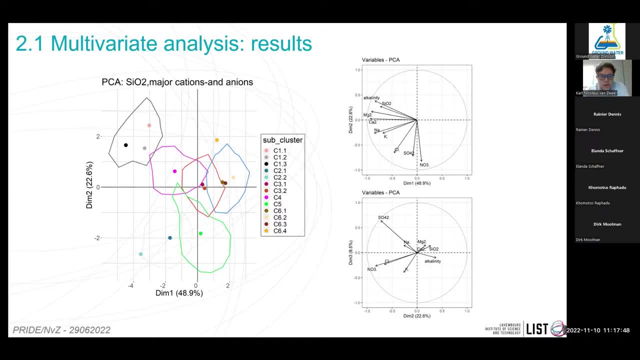 but i'll go into more the chemistry because i need to sort of explain this just to show how we did the modeling. so just to get back to the pca, so what we could immediately see is that most of the the variance on principal component, one which explains 48 percent of the variance in 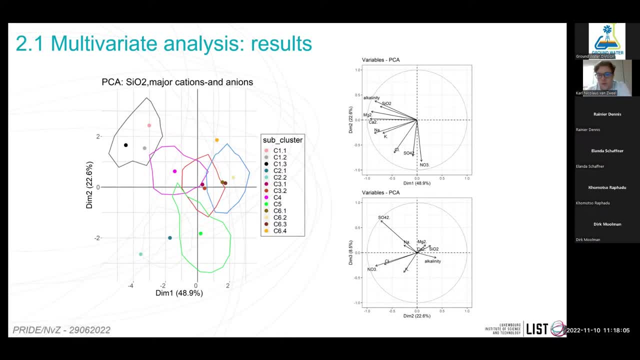 data is just calcium and magnesium, and then also, to a less extent, alkalinity and silica, and then, on principal component two, you have uh sulfate, and then you have a sodium and potassium- i will explain in a moment- and chloride and also nitrate on the secondary uh of the pca2. and then if we compare uh pc3 with pc2, you can also see that 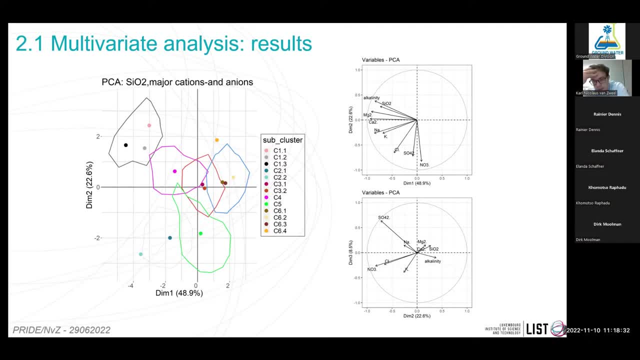 there you again see calcium and magnesium, and then and, and in this case what is interesting to note is that sulfate and alkalinity sort of have a inverse influence on the, on the variance, and this i will explain in a moment. so if we then again look at the, the piper 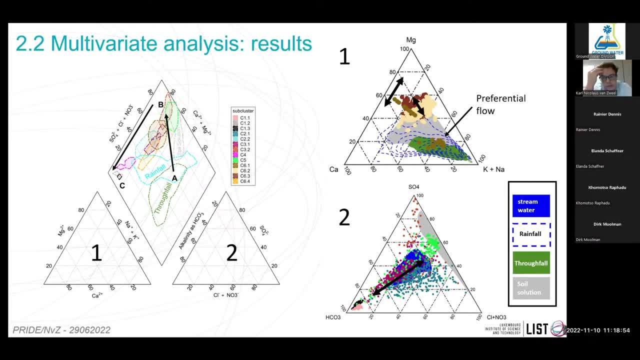 diagram, but we sort of take away the dots and we just look at clusters. um we we can look at the ternary diagram. so we can discuss ternary diagram. uh, one first, which is the cations. uh sorry, uh yeah, the cations. so what is interesting here um is, uh, this a gray area. here is 500 um. 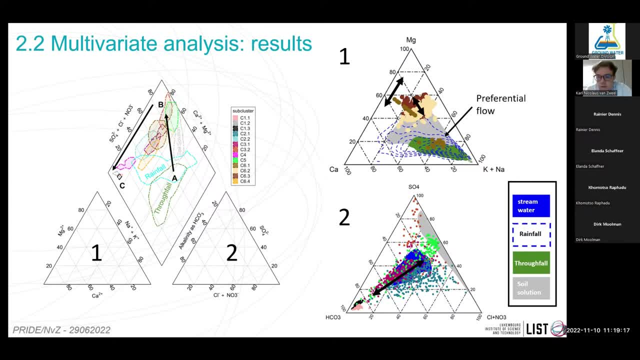 soil, water data points. so this forms, uh, this really distinct uh area. and then what you see here in the, the sort of uh green color, the um is uh, the through fall influence, and then the blue contour lines is the rainfall. so these three components make up most of the shallow ground. 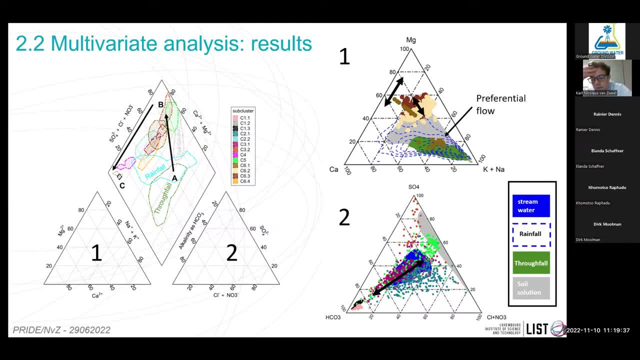 water. um, because we have a lot of preferential recharge in terms of a lot of rooting uh the the uh transformed water streams- equal soccer bottom year 야. the deep sections and the uh uh underground Pe squat the the раньшеyt to that here and thenの the decided and This 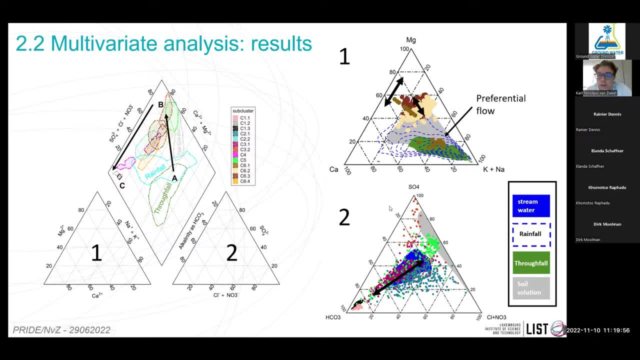 also gives some of the Anfang boundary points. and there's one more. Hopefully it's not really a super yummy ㅎㅎgoed, but it's the interesting Periwardal theme here, Because it's so interesting. uh, so we observed, so you can think the Fig리 can be well optimized to. the deep sections. inți cò saved inÇ. so they sort of bypass the, the organic horizons of the soil and go directly into the mineralize shows, so by the to shallow class this. this is what is interesting, that we observed in this way- or is the ministry but we could not explain sort of. the difference between the two is that they have more or less the same variance in terms of calcium and magnesium, but a but a distinct difference in terms of sodium. uh, a considerable, many. 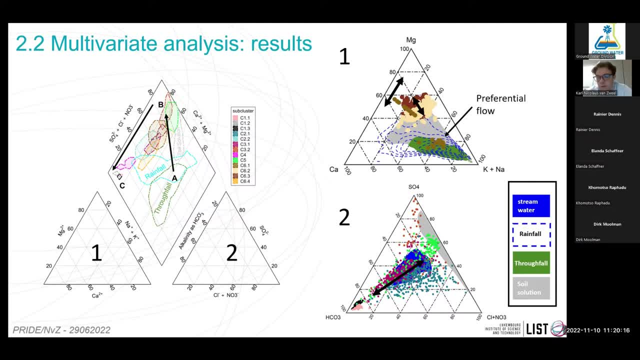 concentration compared to calcium magnesium, and this is solely because of iron exchange. so what happens? there's this sort of light, uh color, uh cluster. it is in in when it is dry, you have rapid infiltration and you have vertical flow through the swell. so not a lot of iron. 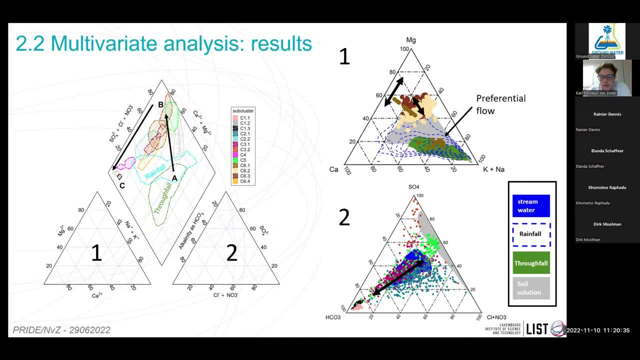 exchange takes place, but in the wet uh uh, when you have, uh, when the system wets up, you have lateral flow through this horizon and you have a lot more iron exchange. so then we can already distinguish these two um clusters from each other, just in terms of looking at iron exchange and then looking 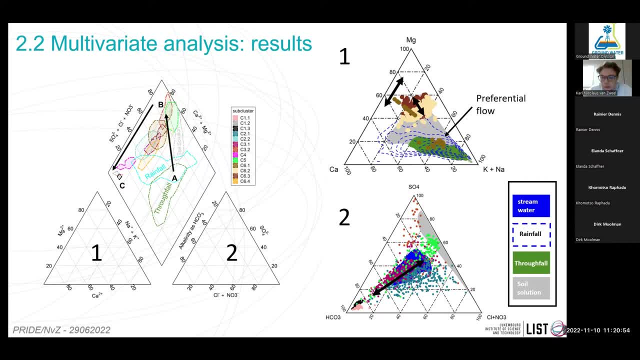 at the anions, we could see that again. this is the soil, uh, water here, and this is just the clusters that we observed through our archaeological clustering. there's two clusters here. this sort of pink and black is the deepest clusters and, as you can see, most of the 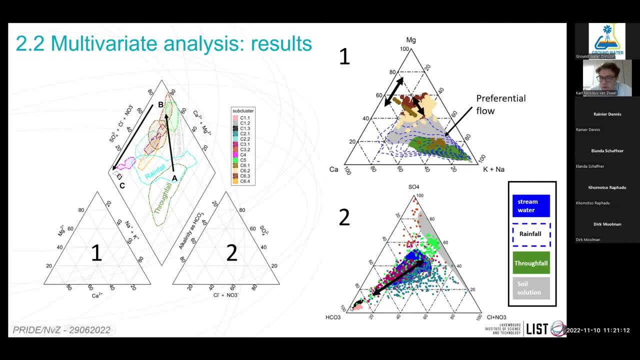 the groundwater as it moves deeper it sort of converges to the deepest point and the blue that you see in the background is all the, the surface water samples. so it's about uh. now data set around 3 000 surface water samples, uh samples that can make this um, this area here. so you can see a lot. 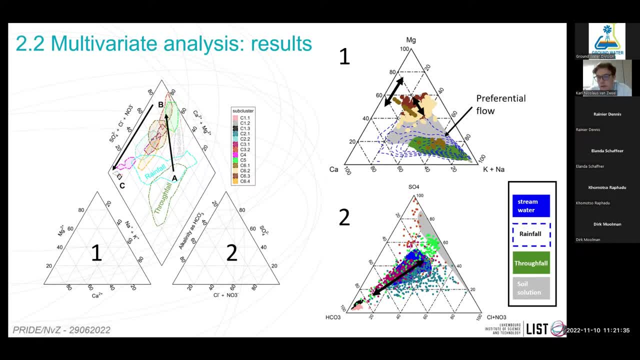 of the time, the, the surface water, is just a linear combination of this, um, this clusters that we observe uh, but uh we can observe in members in the system and this is what we're working towards. so, explaining what is happening and why this uh trends are occurring, is what the geochemical 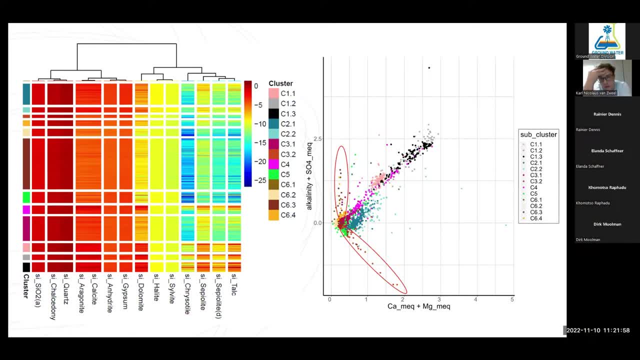 modeling is all about, so i'll discuss this a bit. so in um, in the database it was around 3 800 samples, that at full um. full uh, all the data so i could model this and freqci uh, model um. i didn't manually input everything which you can do it in python on arc. 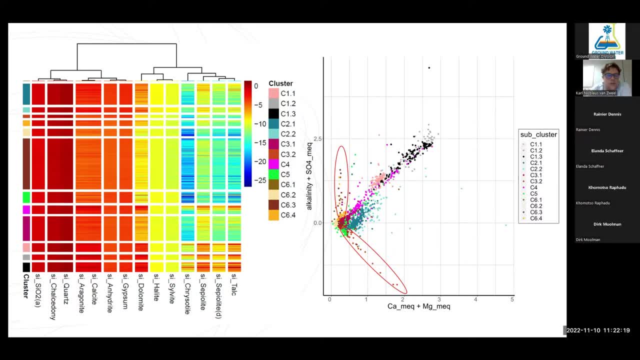 um, so i ran uh this, uh the data and to to see what uh outer saturation this is of the minerals. look like, um, and what we could see is more or less what we already expected is that most of the the anions are are controlled mostly by bicarbonate minerals. so you can see in the deeper. 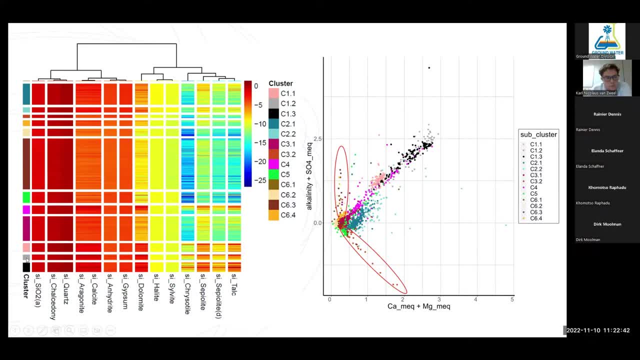 this year, for instance, 1.3 um, 1.2 and 1.1. you have a relatively high saturation in this for dolomite and calcite and then also for gypsum, but gypsum is throughout the system um. i did not show the xr dnx of f data or results that we found, but we more or less saw a lot of this type of. 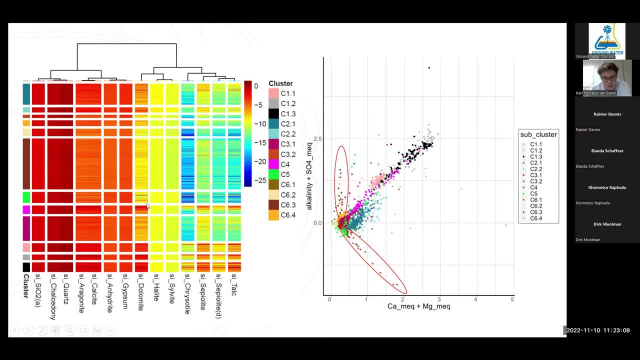 sulfate minerals in the system. so anyway, when you plot the raw data, the calcium plus magnesium equivalents against the total alkalinity plus sulfate, you can more or less explain most of the chemistry in the system, except for two sort of- uh, special cases, and this is what's happening in the riparian zone and i will discuss. 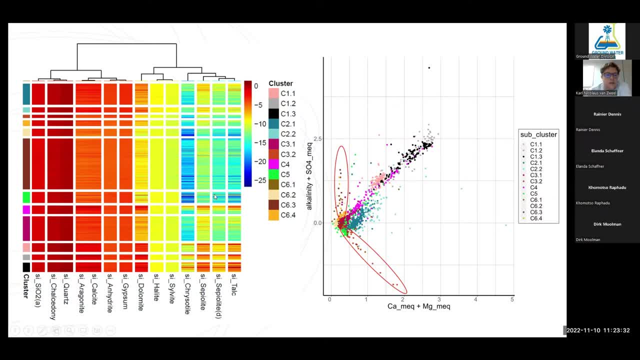 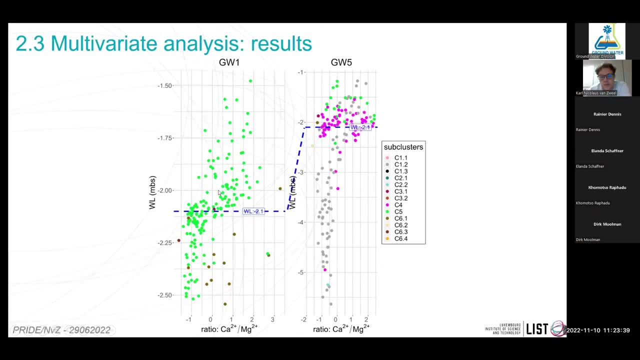 this a bit later. so this heat map really gave us a good insight into what minerals to consider in our model. so, uh, we just again check if the, if the clusters, make sense. so this is a water level versus a scaled uh, z, transformed calcium, magnesium, racism, meaning the mean is zero and the standard 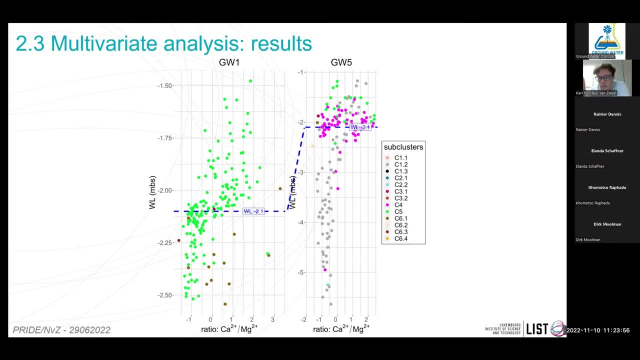 deviation is unity, right, so it's just the scaling so that we can see the variance between points and this. you plot against the water level and you can actually see. it's quite interesting. so this is quite a performance model. so this is what i can see. is we have a? there's a more? uh, 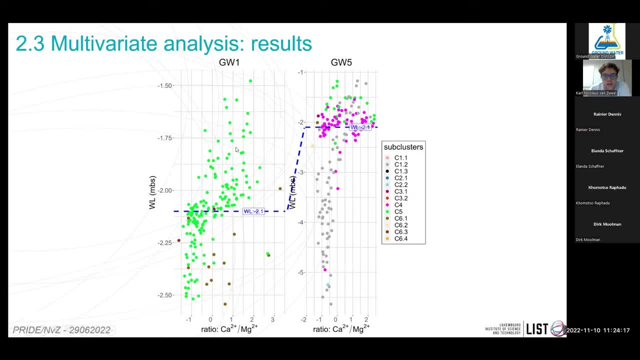 cross-dtag one that's at about 2.0 meters deep. so that's a very important information. so we have two types of uh subsets. so you could see: uh, this is a glass and the very bottom is the bottom. there's a little more uh, right level. uh, this is a solid well below that. so gw1 is a. 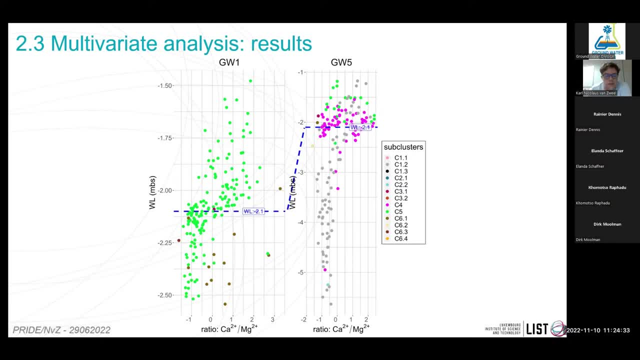 shallow. well, it's about 2.5 meters deep and just next to it there's another. well, that is notice this sort of validated our hypothesis that we could see preferential flow paths in terms of chemistry, so when gw1 is really dry. so what you're really just pumping out is, um is just see pitch. 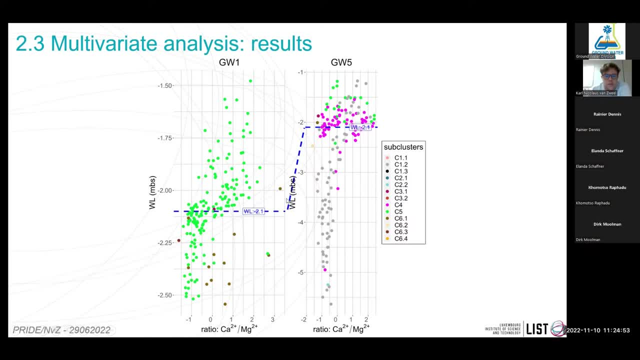 from the top you can sort of you see the, the, um, if there's rainfall events, you see the bypass. so the, the water is not the, the recharge is not chemically altered by the soils. it sort of just bypasses and gets into the deeper part of the aquifer, or relatively deep, in two meters. 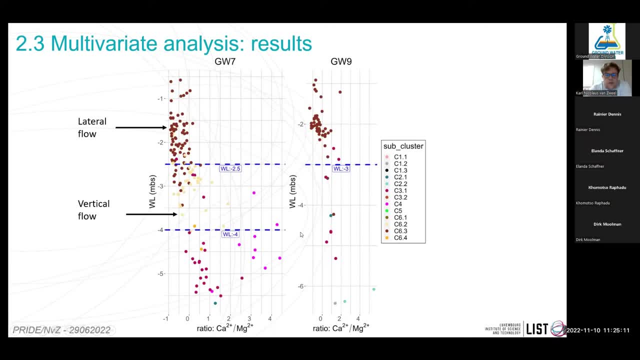 so on the on the slope, this is now below the weathering front. so below this sort of elevation where the the weathering front stops, you can see you have a bit of different chemistry. so here you have a very um, you have the the slope, so and there's just really the 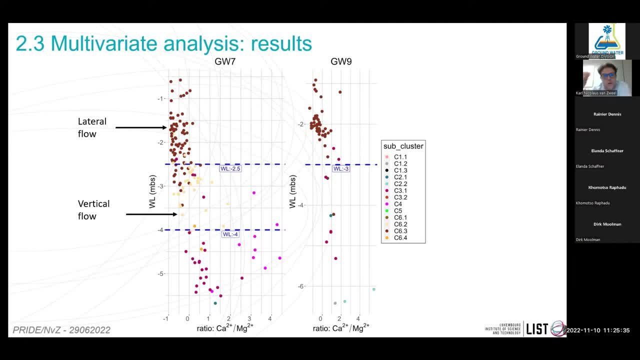 bit of weathering on the on the bedrock. so when the system is really um wet, you see this lateral flow line cluster that we observed also in the ternary diagram, and when it dries out you start seeing that you have vertical infiltration through the soils and changes the chemistry right. and if 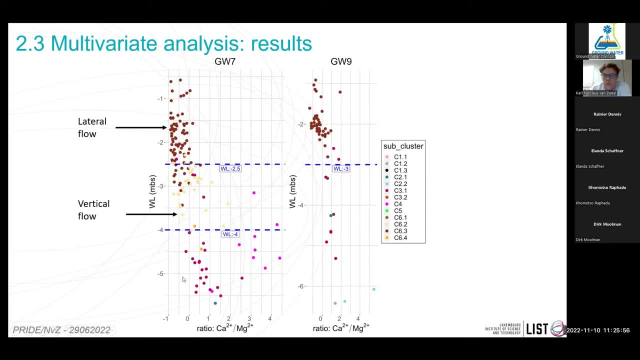 you move in deeper you start seeing the water that really provides the base flow to the stream. and then this purple cluster that i had, that i showed you that mostly is formed on the plateau. um you, you also observe this on the yield slope. so what happens is that the, the yields on the plateau, you have sort of like a quasi. 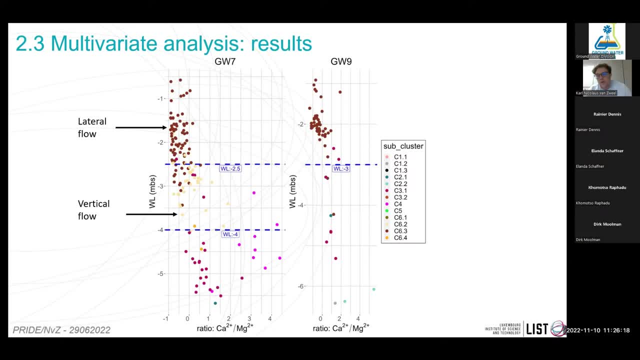 perched aquifer situation. so you have this weathered material that's sitting on top of sort of a sort of semi-leaky or fractured slate that is quite dense. so if the water level goes up to a gold and it sticks in between the two, the soil flow also distinguishes in a gra reasons you. 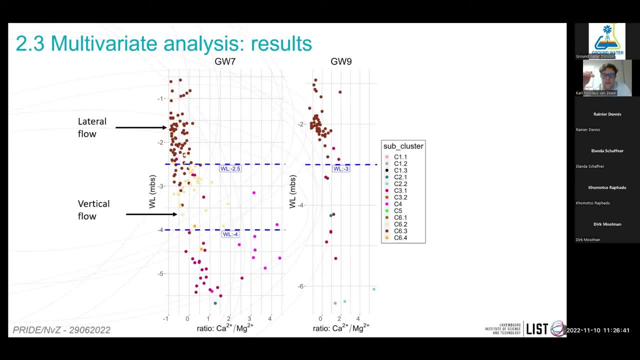 can see on this yellowish orange that that initially- but let's put green throughout for now- that earlier in the distance comes out and then the different flows are going to press eventually, and then the yellowish, brown and yellowish green fall further. at an average degree that Dilraha has, we can see a nice hard取tho and another red. никаких mine, in fact. 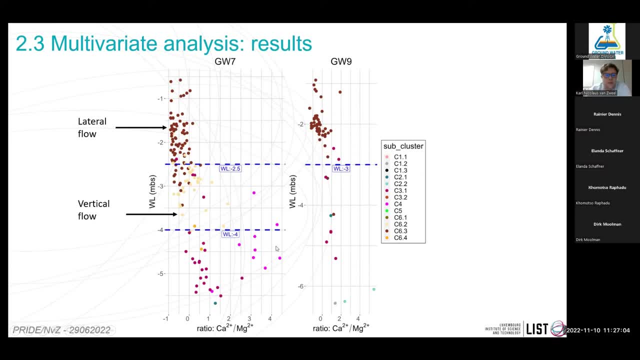 is just a gray syringe right there, that's a talked about on the bottom of the slide with those two. so therefore we get 4 meters deep into the soil, soil waters and the sort of vertically infiltrating soil waters, and this we could also prove through mixing models. so, because this you don't see in the stream, but we could. 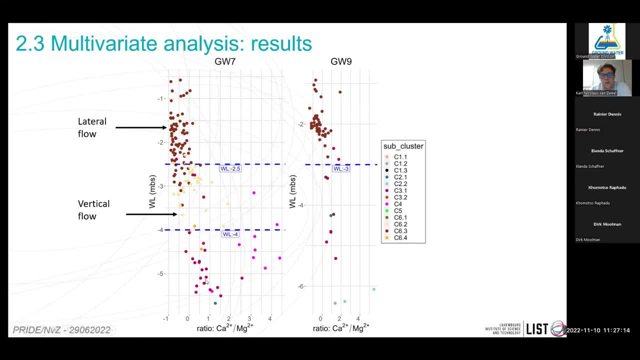 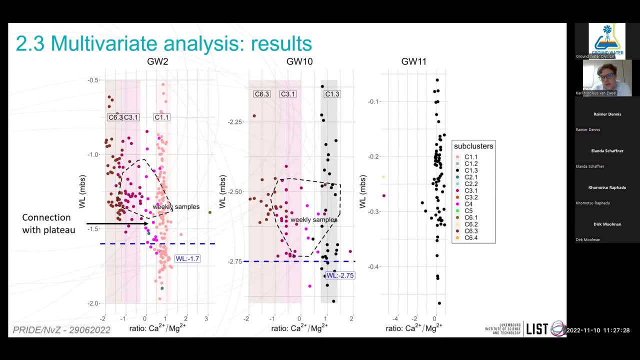 see that this cluster here could not be fully explained by just mixing these two. we had to add more sulfate and this is produced on the, on the slope, on the plateau, sorry- and then just near stream chemistry. so this is quite close to the stream. on the outlet you can see sort of all. 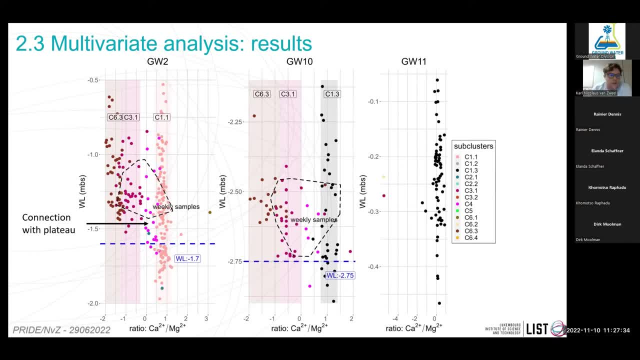 the flow lines converging. so you have this, the shallow, shallow flow line. and then you have this mixed flow line that is comprised of the purple cluster and the brown cluster, so most of this goes into the stream, and then you have a deeper flow line that is formed on the, on the slope. so 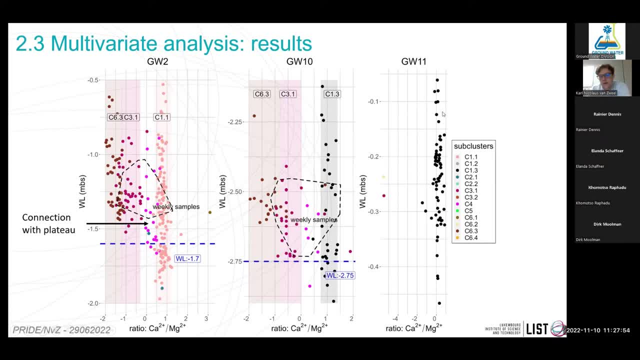 it's not completely the same as the deepest flow line that i showed in the initial schematic flow line d. it's a bit younger but still flows through the in system. so this more or less validated that our classifier picked up or really did a good job at. 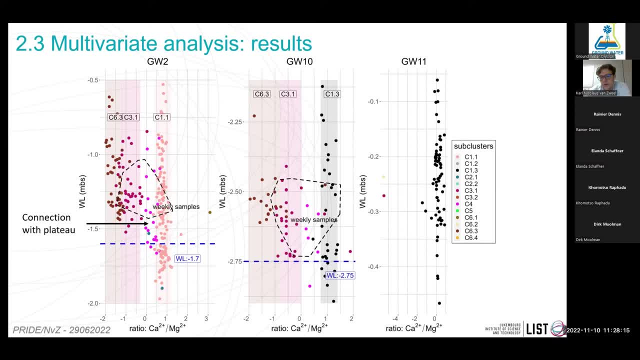 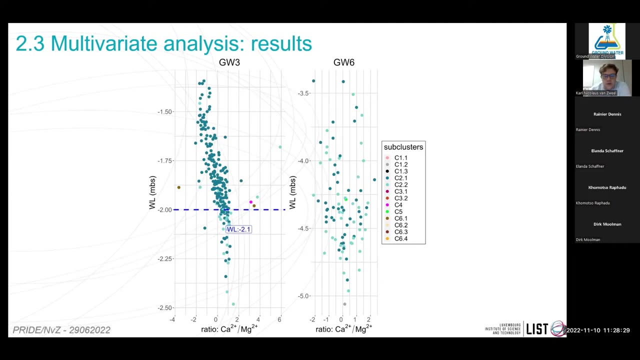 separating the water signals that we observed in the sampling and then we could start trying to model with this. this classes, right. so just this is just interesting behavior from the secondary plateau, because there's such a shallow weathered front and it's highly fractured most of the, and also it has a different type of vegetation that we see. 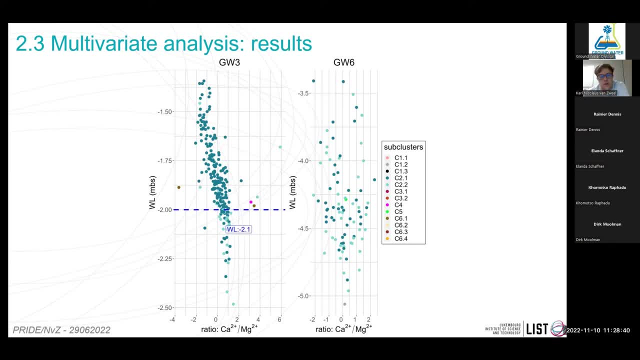 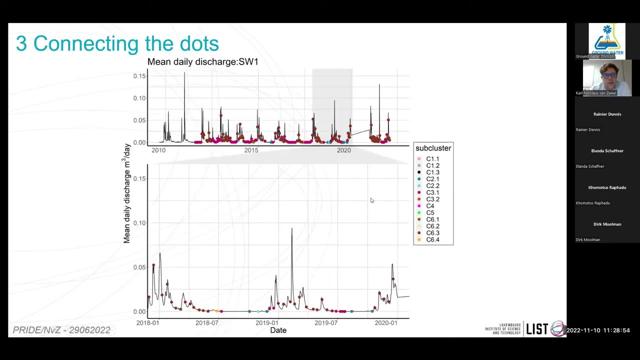 has a lot higher input of nitrates and chloride. so you can definitely see that it's chemically really not altered, it's just recharged, runs through the fractures, fractures and is discharged into the stream. so just to show you quickly what we now did, is we sort of every time we add a sample. 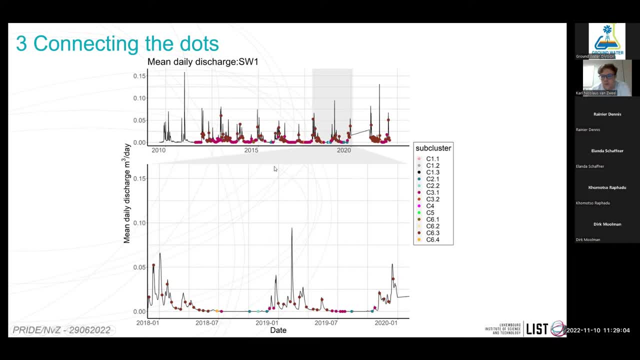 we plotted this on the daily discharge of the four um four stream flow gauges that we had so and then you can actually see it works quite well. so when you have high flow it's just a shallow stuff. this little point here is what i'm currently working on. this is the chemical alteration in the 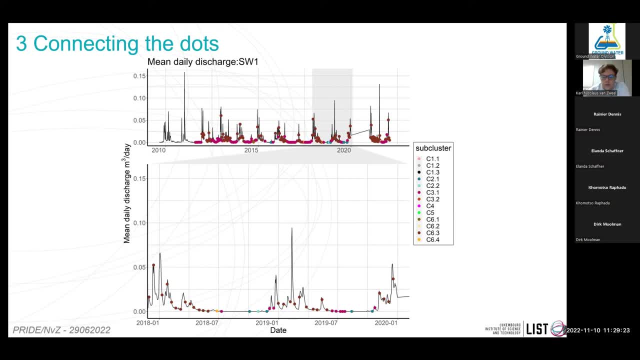 riparian zone. so if you have dry conditions and you have a small rainfall event, the first peak is usually just water that is stored in the riparian zone that was chemically altered a bit. it gets pushed into the, into the stream, and then you see some of the deeper flow lines. uh, when it 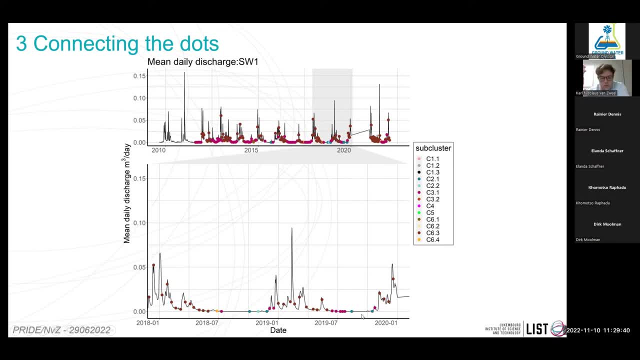 is really dry. uh, just to to also give you a bit of background, our catchment dry. the stream almost dries up completely in summer. this is due to the fact that evaporative vapor transpiration plays a large role in in the water dynamics of the of the system. so, um, you can almost have a 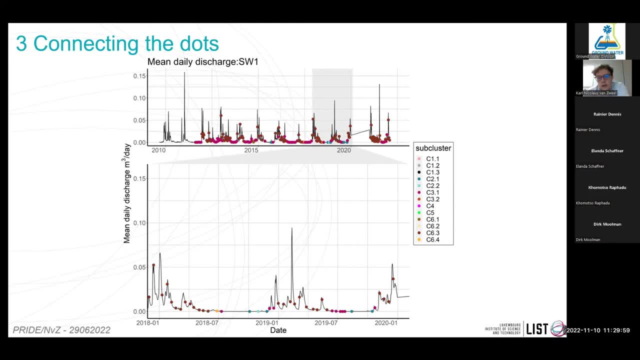 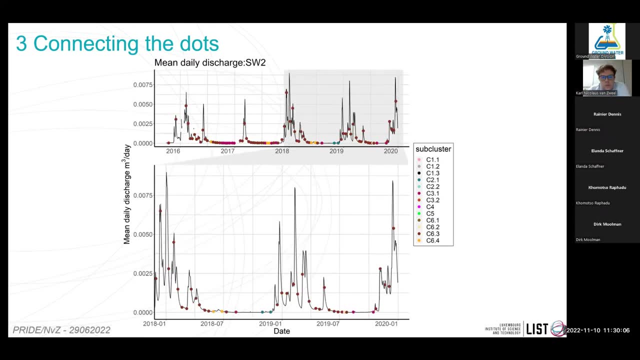 completely dry system in summer, where there's almost no water, and then in winter it fills up again. um, so then sw2: we saw more or less the same sequence. so this again validated for us that our clustering method really worked well, and so the next step is now to really 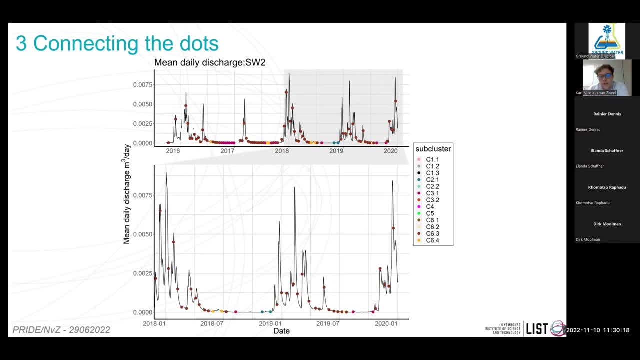 see if the clusters we observe are they true in members in the system or are they linear combinations, meaning that are there mixtures, uh, between between clusters? uh, because at the end of the day we aim to do what is called a string flow separation, and usually it's done through stable isotopes, but you can also do it through 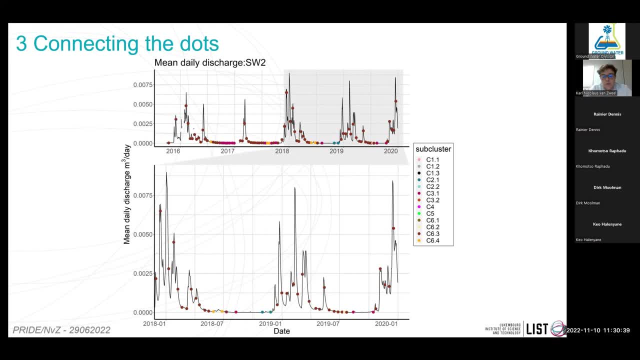 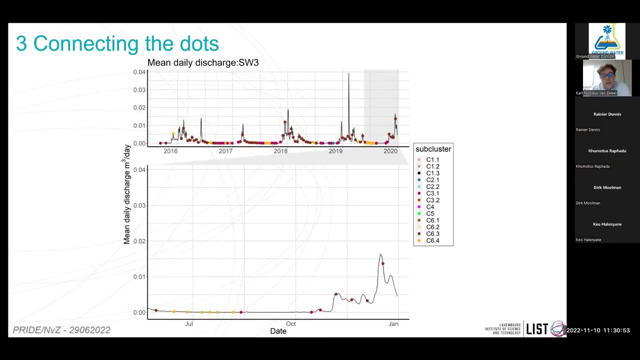 chemistry. but you have to make the assumption, really, that you have a conservative tracer, which is actually not the case for most solids or natural traces in a system. so you have to separate the mixing variants from the chemical variants, right? so this is the aim, then, is to account for the chemical variants and then 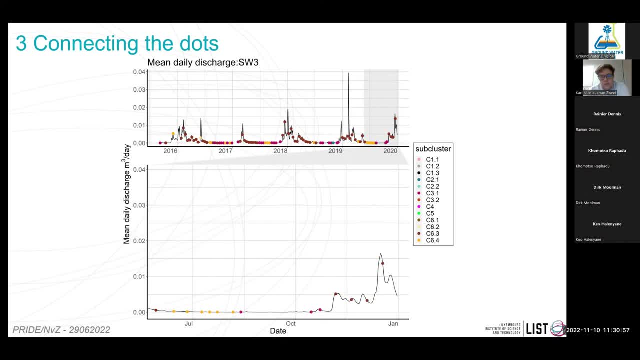 we can. what we left with is mixing variants and then we can start understanding what generates string flow in the system. so this is the last one, sw3. it is situated really close to big riparian zone, so you can always see and dry periods, the entrance of the riparian zone, but for the most part is dominated by 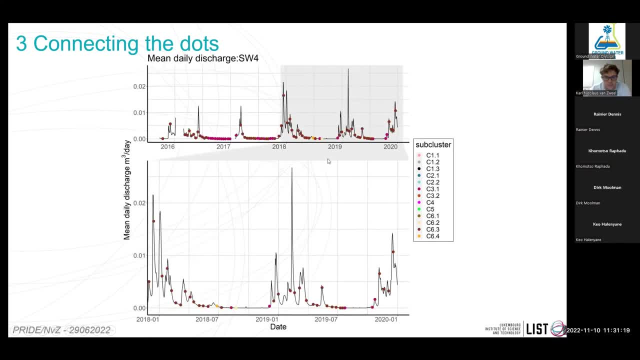 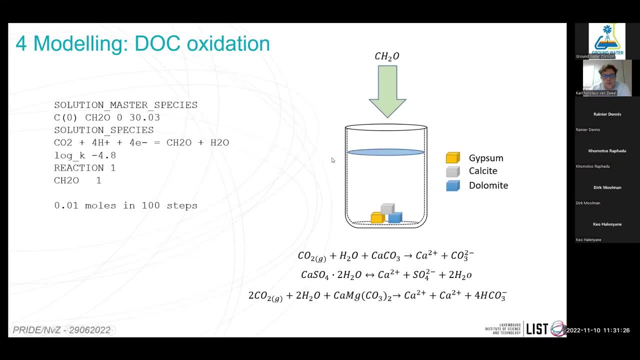 shallow flow lines in high flow or wet conditions. the last one is sw4. same basic story. so we are fairly confident with this results. so we will go now, sorry, to the modeling of our own result. for us this is the whole July: the earth itrailth home, which we we also found in. 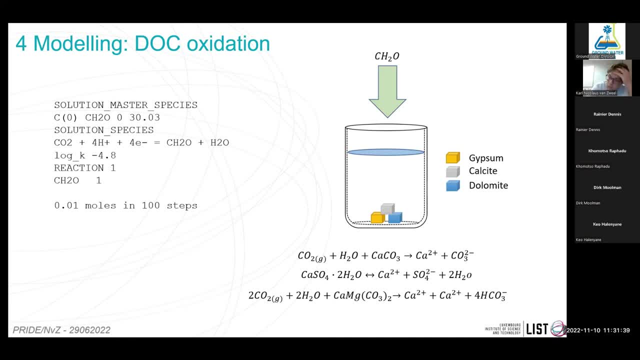 mc2 ut safely in utopia. this is the moment we finally wanted to be able to see、、 the. the earth fit very perfectly and you can see that it passed almost everything in the system so far, but we're still in a state of we moving, but it, the, it is not in the system. 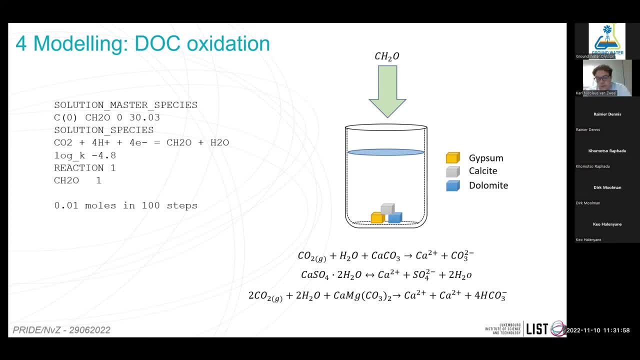 and so it's not really fixed at all. gentle motor up and down, but notiggles, or so I'm sort of certain about it. so we hypothesized when we said, well, okay, there's a lot of dessaHEA system, so, and potentially we didn't, we didn't pick up any pyrite in the mineral. 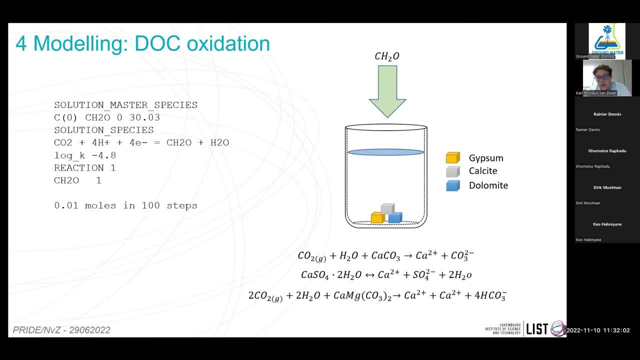 and vegetation cycling. this includes sulfates. the sulfates can be reduced in summer to pyrite. it gets oxidized and so it's a sourcing situation, or it can just be stored as calcite, because this is also. maybe there was pyrite, because the weathering front on the platter is about 20 meters deep. 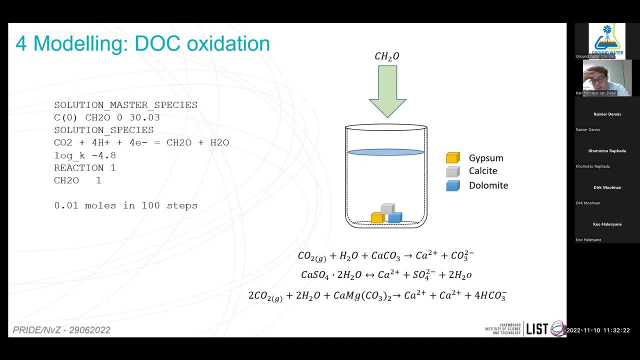 and it was stored as calcite and it just sort of leaches out. because what we saw in the in the throughfall is it can potentially account for the sulfate dynamics that we see. but on average the mean- the mean sulfate value- is relatively low, about 2.5 milligrams per liter and the highest 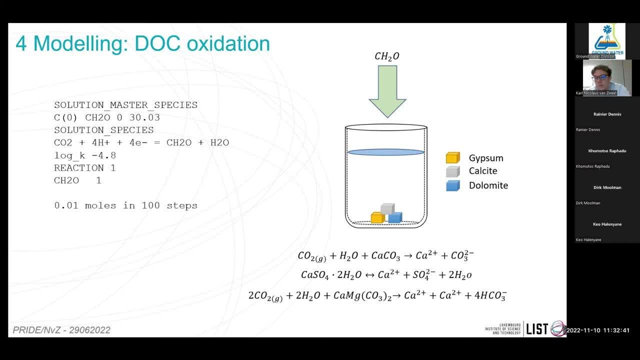 values that we observe in the deeper flow lines are about 14 milligrams per liter. so there has to be some source or at least some temporary storage of sulfates in our system. and then we also had to account for the increase in alkalinity, so basically we could state that, okay, so the the primary proton donor in our system can be pyrite. 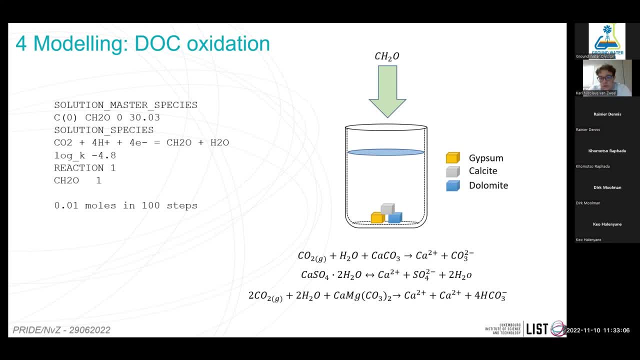 or it could be just oxidation of doc salt, organic carbon. so to do this we can do a virtual experiment, right, so we can say: okay, say there's no pyrite in the system and all the sulfates are stored as calcite, as gypsum. sorry, and we know that in the system we have calcite and gypsum. 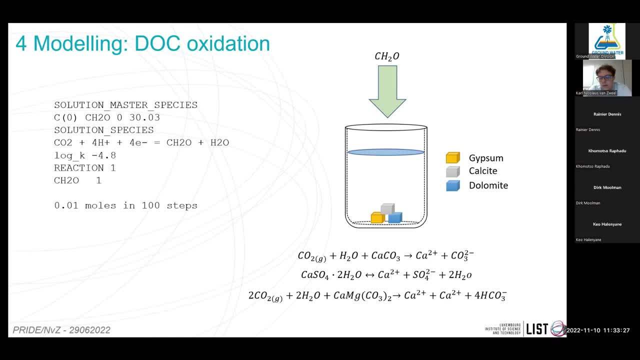 and you can have a complex, the, the dissolution of calcite can also drive the, the dissolution of gypsum, for doc. oxidizing it forms carbonic acid, so it's just a sort of restoration. so we can test this in 3c, right? so we can start by just saying, okay, we, we take gypsum calcite and there's also magnesium. so 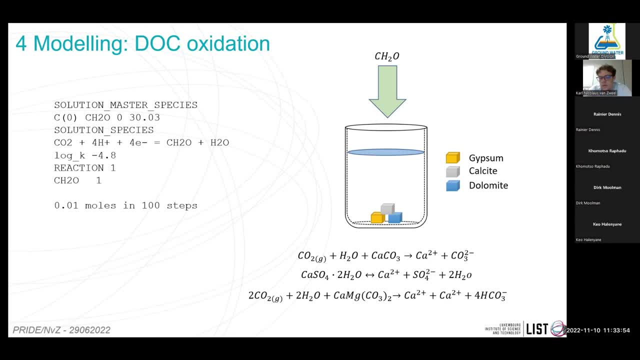 the question is really: is it dolomite or is it magnesium calcite? we don't know, and it's quite difficult to model magnesium calcite for this. so for the future, we're going to have to do a little bit of this exercise. we'll just take a dolomite um as a proxy, so a mixture of calcium. 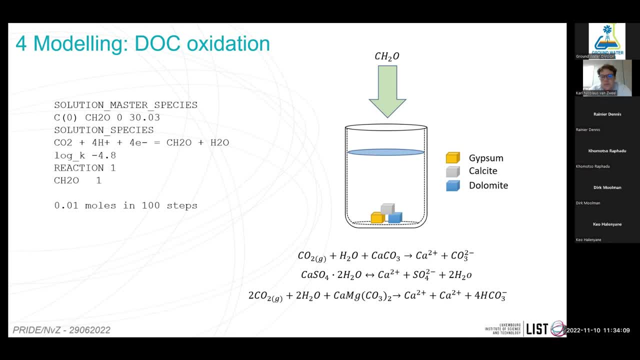 and dolomite would probably explain our calcium magnesium dynamics- and we add some gypsum and then we sequentially add doc. so in this case we doc for us is just acetate and we oxidize that. we add 0.1 moles of- sorry, 0.01 moles of acetate and we see how the ph changes, right? 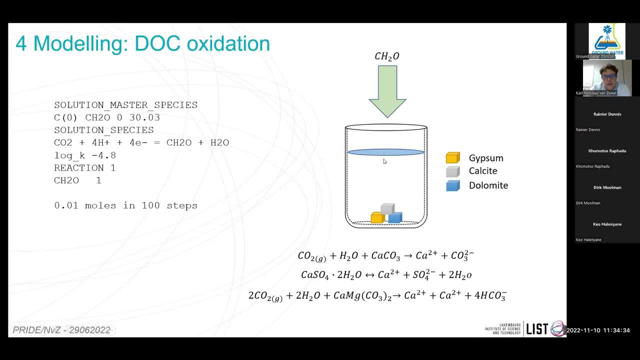 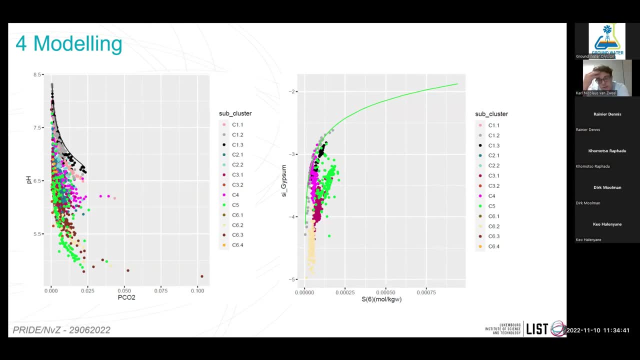 so this is, if you visualize this, just a little batch exercise. so this more or less explained, uh explained, the the deeper flow lines. actually quite well, just doc, because we see a lot of doc leaking into the deeper stuff through preferential flow paths. so, theoretically, if you have homogeneous 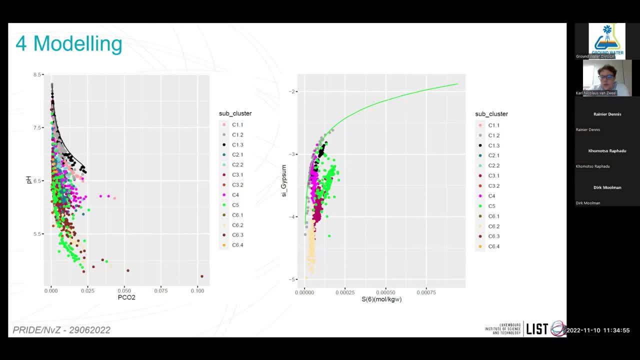 porous media, your doc will be oxidized way before the time the water arrives or recharges deeper. so you have to have preferential flow paths for that uh to get the doc down there. and this more or less explained what we saw. so pco2: here is the partial pressure of co2. so for those of you, 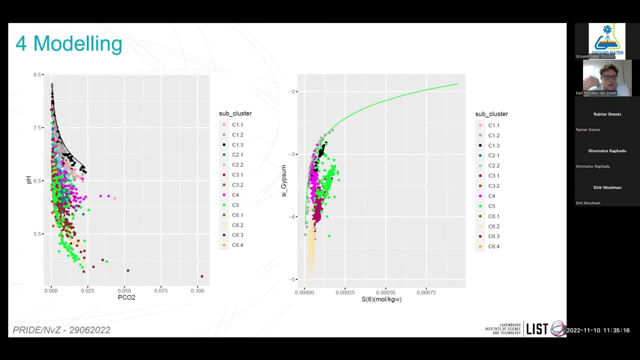 might not know how to how this works when you have a doc that are that is oxidized as a combustion reaction. so you have co2 that forms as a product and co2 as a gas then dissolves into the water, forming carbonic acid and the. the amount of carbonic acid it forms is a function of the, the partial pressure of co2. 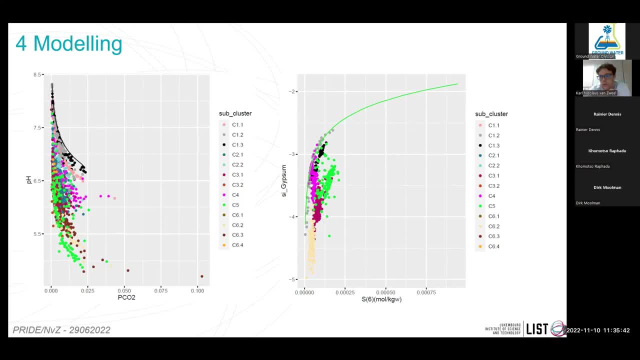 and also the temperature, so you can look at the injuries laws, just how much gas can then dissolve and form uh, carbonic acid, and the carbonic acid then drives the dissolution of calcite because it's just a buffering right. so theoretically then, if you measure ph and you know the total, 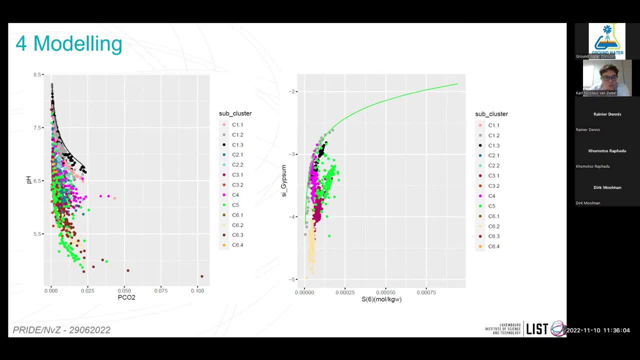 linearity you can calculate the partial pressure of co2. so i won't go into uh, into that too much, but you can go read about it. a good reference i can suggest is a book of tony uh of apple and posma. it's like the g chemistry bible for me, but a really good book anyway. so you can. so what you? 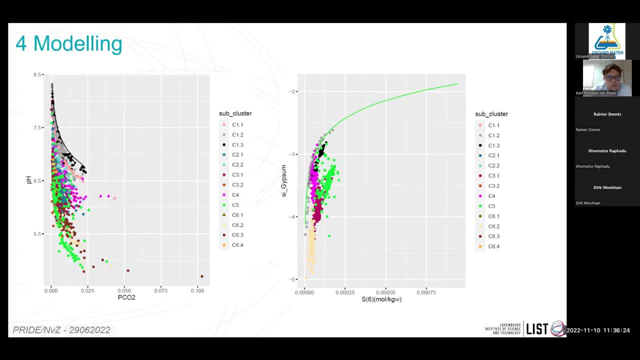 see, here is the clustered data modeled in freqc. so and then this is this black line. it's just my little batch experiment to see if it could work. so then we theorized: okay, doc, can probably explain most of the the ph behavior that we're seeing in the system, and uh, you can. and the model also effectively, uh, or really effectively. 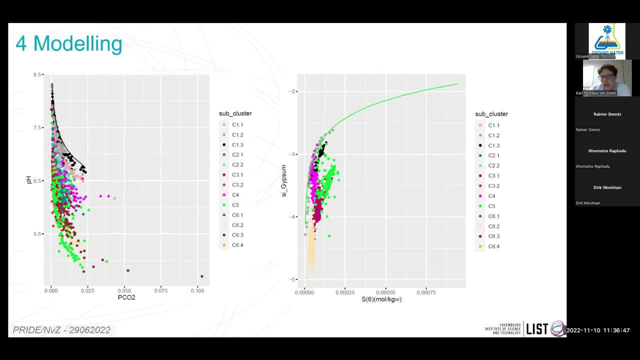 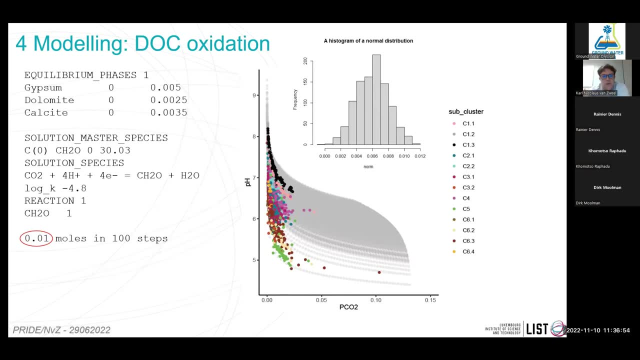 predicts the, the relation between gypsum and sulfate. so what we did then- we said okay, well, obviously, um, the, the gypsum and the calcite and so on, was, uh, you can't just uh estimate the parameters. but you can't just uh estimate the parameters, but you can't just uh estimate the. 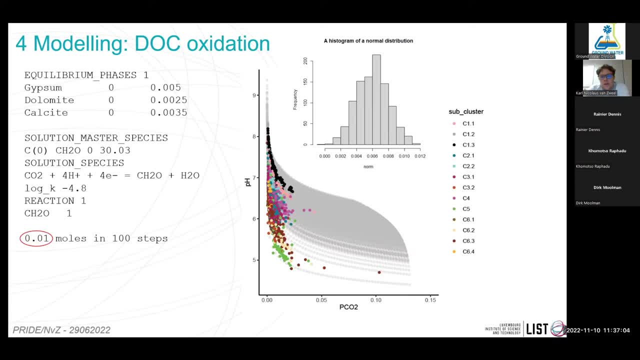 parameters. but you can't just, uh, estimate the parameters, although you can get some data on the segment by testing the ERROR 0K, the acetate. that gets input at various depths and you just run a sequential reaction model for it model. but it's sort of a small sensitivity analysis. so you basically take. 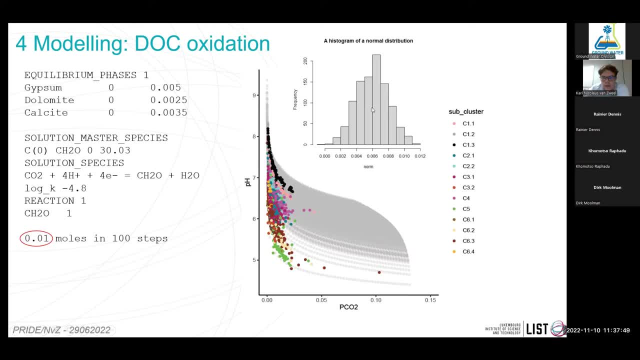 every time a point that has the highest ph and you titrate it or you add acid. right, we could more or less explain what is happening in terms of the phps co2 dynamics. so this gave us a good. it showed really positive results in terms of a monte carlo simulation, which was really well. 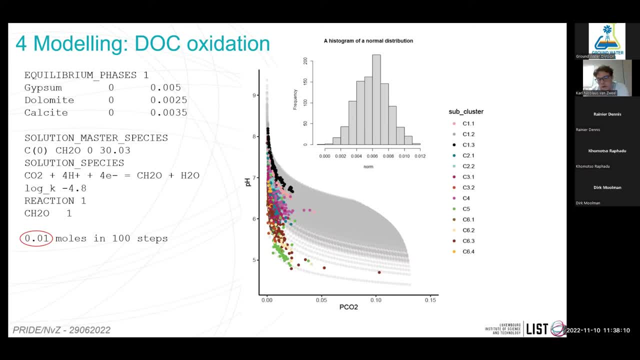 to to predict the dynamics of of uh, sulfate, calcium and magnesium in the system. so how to go about it? well, i'll just quickly show you just inside a pixie for the guys that do know. when you have equilibrium phases and you tell you constrain the system, you tell the system okay. 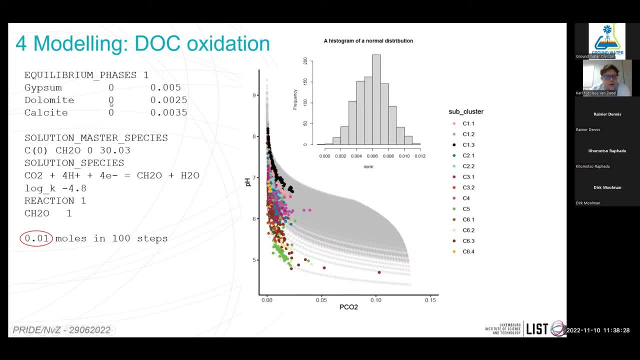 you want calcite, dolomite and gypsum to react, and until it reaches equilibrium. but then you can also calc. you can also define the amount that you add to the batch experiment. so in this case, if you make it 10, there's ample and it will reach. 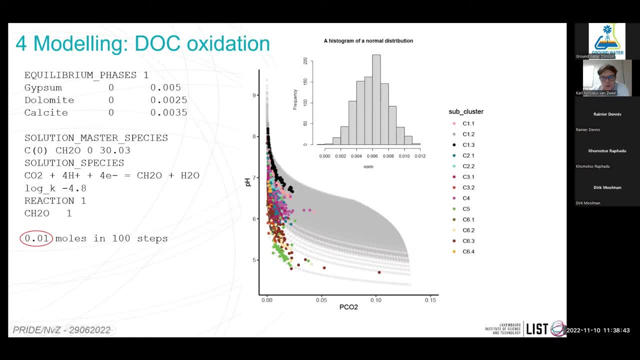 equilibrium. but if you make it sufficiently low, it will never reach equilibrium um it. but it will try to right. so it will use up all this moles that you define for it, but then it will try to get to equilibrium, but obviously you will not reach it because there's not enough reactants. 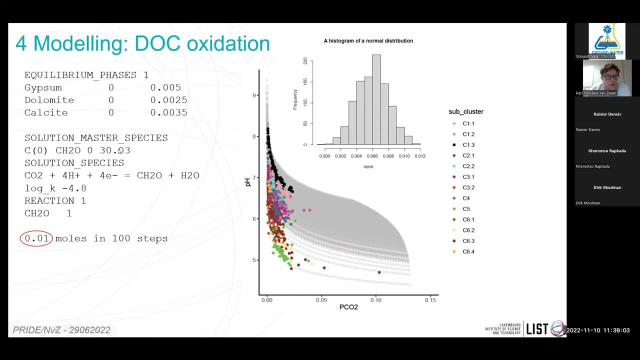 when you add uh, doc, okay, so you have to define doc. it's not in the, the default tricksy dot that database, perhaps it is, i can't remember, but it doesn't matter. you can um. you can just define the kinetics, uh, or the thermodynamic parameters yourself, or there might be some other um databases. 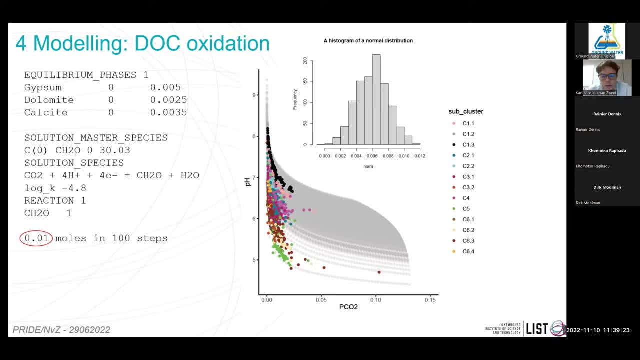 that might contain it. but you can do the same by just uh varying the pco2, so the, the partial pressure of co2 under equilibrium phases, so anyway, so this model more or less uh worked well, but the problem is it that did not predict the the sulfate values really well, because in effect what it does is it takes, takes a point. 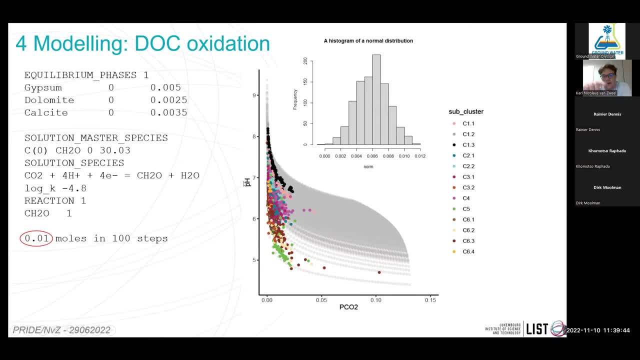 here and it reacts it sequentially, so you add the sort of weird lines going all over the place. but what we could do then is, uh, we could do away with the sequential modeling and just vary the pco2, because we know this is related to the acetate. 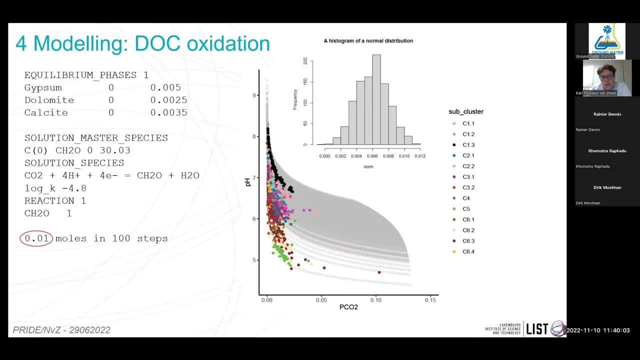 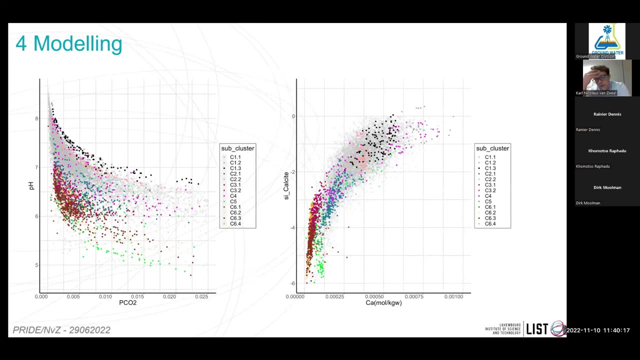 or do co2 oxidation. so if you then have the normal distribution also for the pco2 and you've also the distributions for for gypsum, dolomite and calcite, uh, you can run a monte carlo simulation, and this i did in frixi, but with r, and i will show you in a moment how you can set this. 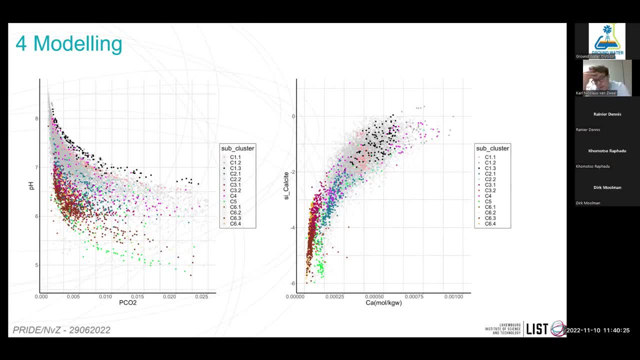 up, but um, running ten thousand models, um actually predicted the behavior really well. this is the ph vs pco2 which you can see it, um, it's relatively accurate. i haven't calculated the errors of the model yet. this is what i'm busy with now. it's uh, not, it's not always that easy. 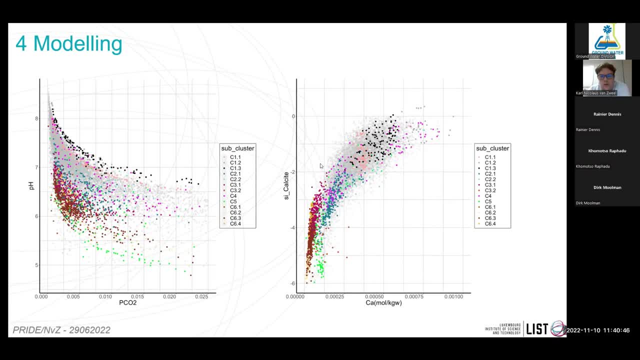 to define your competence. so in the model with monte carlo, especially if you have a lot of parameters, um, but for now it looks really promising. and then also calcium. this is calcite, it's just uh, it's really fairly uh nice results, as you can see there. so the gray light dots in the background is my models. 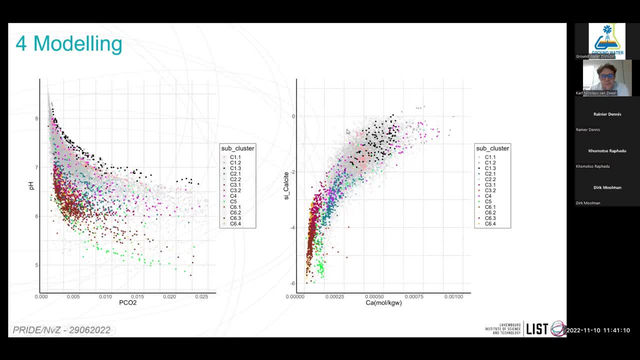 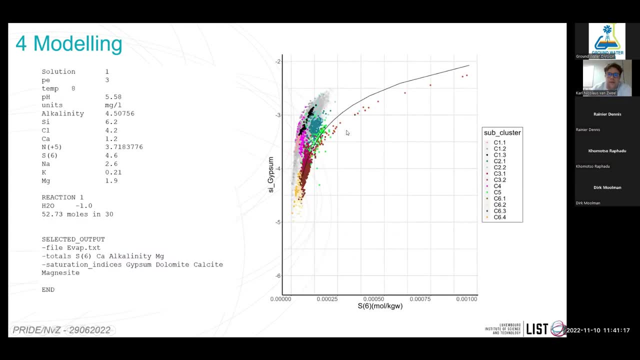 and obviously the colored dots in front is the sequester to be identified in the system, and then, uh, in terms of sulfate. so this is where it gets a bit interesting. so we could pres, uh, we could predict whether sulfate is coming from riparian zone, um and i, so the model could not effectively. 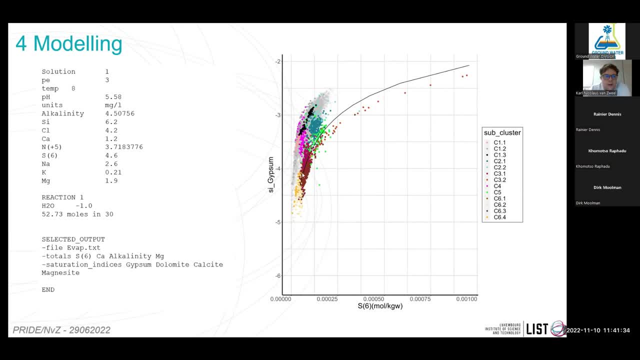 predict the concentrations. but if you just run a simple evaporative model, so you take, uh, the, the shallow flow line, you can take the, the mean, or you can take the, you know the synchroid of the cluster, and you just evaporate water, it sort of. 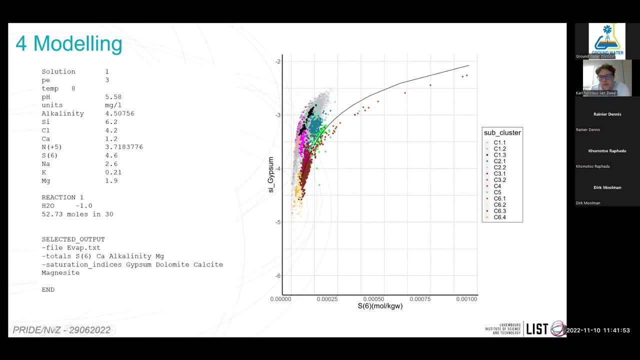 more or less effectively. um explains the behavior that we see in terms of sulfate. um, and then, uh, you know again, this is um, the gray dots on my model and the other, the other colors, the dots are the other measured values. so, effectively, what we could prove then. 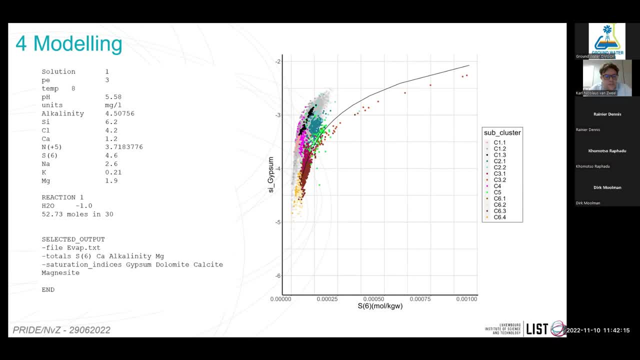 is the pyrite to explain the the um, the behavior of sulfate in the system. it seems to be all coming from uh secondary minerals, so gypsum or anhydrite. so you can more or less model those old system like this and it look that there's a substantial amount of buffering in terms. 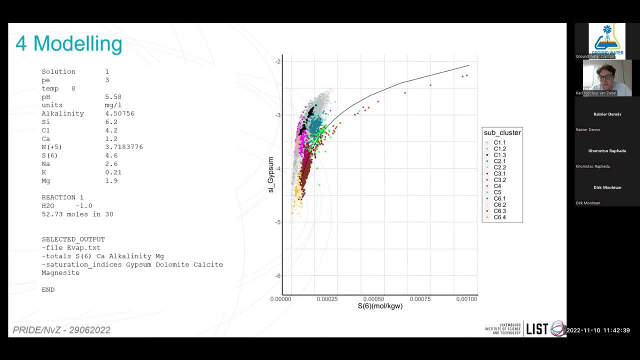 of, uh, gaseous carbon, and so be it for the gaseous principle. it's actually a little bit more more interesting, but the more you look at it, the more it's all kind of very well represented. um, so from this perspective we can call this the pyrite of the濃 and the pyrite of the. 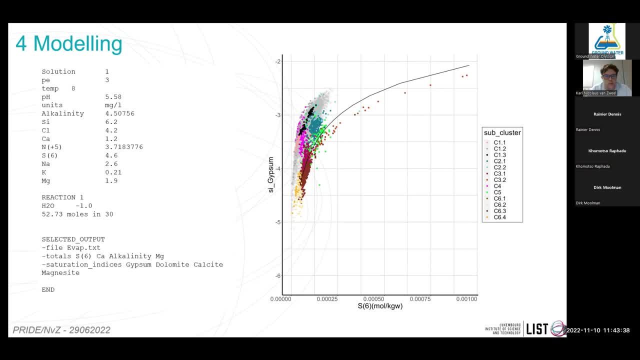 cytochrome of the um. so i'm going to put a little bit on that picture to show you a little bit more of what we can predict. if it's a pyrite, the pyrite like i'm showing you is the silo of a pyrite, uh. if it's a pyrite, uh, then it's in the form of a pyrite, uh, the gaseous character as we call it. so in this case the pyrite is the pyrite of the gaseousreceiver and so it's the gaseous roots. so the gaseous rejoiner is the gaseous root, because it's quite interesting and you can be pretty much. 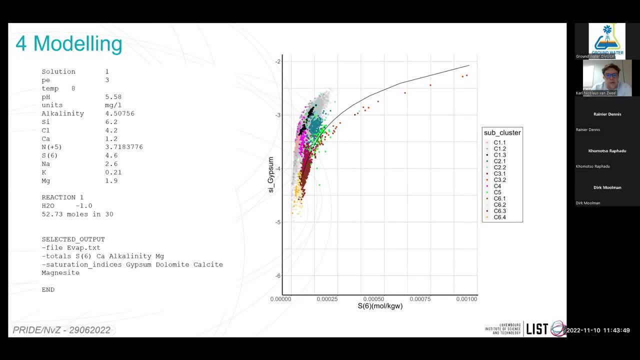 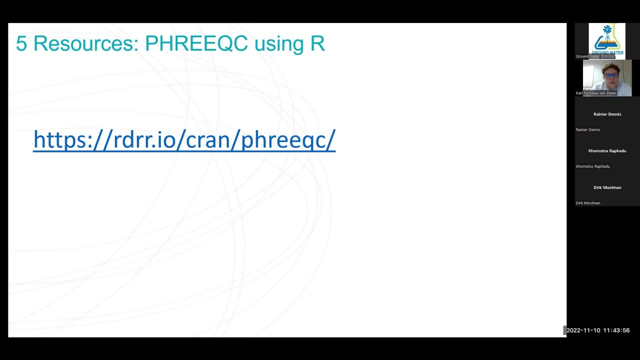 show this today because it's quite interesting and you can do most of the stuff yourself, um, and i'll show you where to get it. so if you for you, the guys that's working in r, which i would now, uh, recommend, i also model in python, um, but it's a bit more difficult to fix it because you have 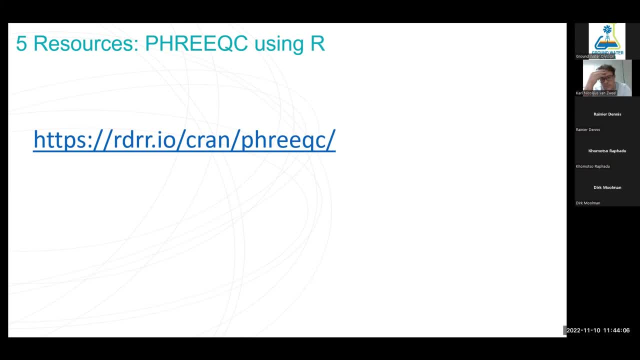 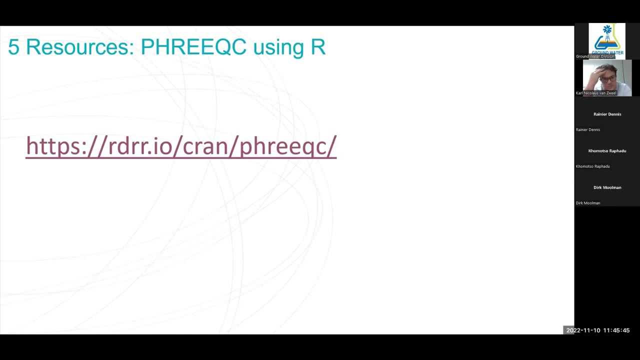 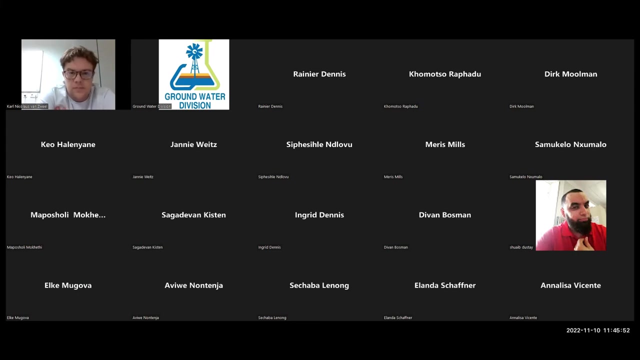 to create your own dll dynamically linked library. you can read about it, just install the library and you can obviously define your, your input file. so the while- well, i think they need over- let me ask a question. so, as a typical south african. um, i see you've got nearly 4 000 samples. 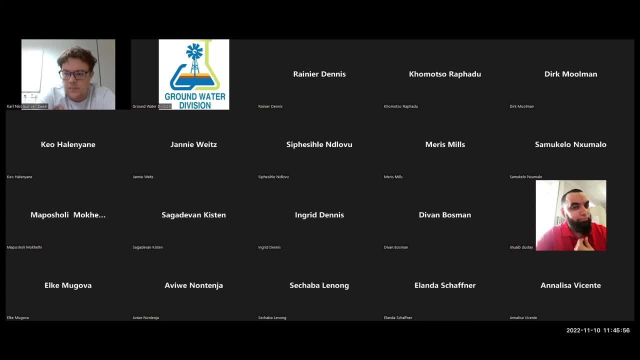 now my question would be: do you think you would have obtained the same results if you only had 400 to work with? because we'll never have the luxury of of of running a project with with that huge amount of samples in the database. yeah, so one of the things. so i just have to also say that it was. 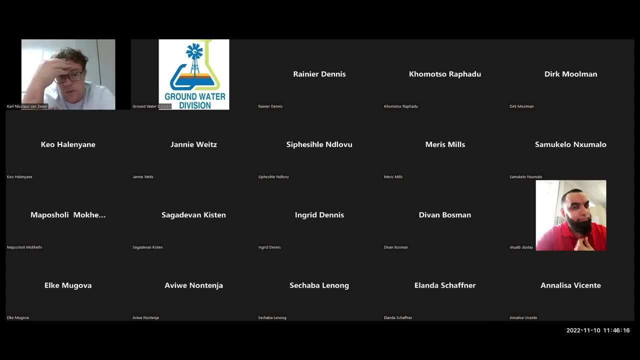 quite a? um big mission. so initially when i started i only had data for three bottles um. a lot of the data, a lot of the samples was still in storage and we appointed a lab technician to to run a sample. so in three years he did 5000 analysis. so i didn't have to the data at the time. so what i did is 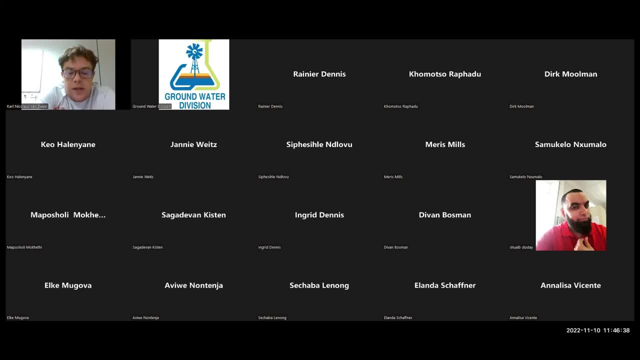 you can also run a sample and then create um synthetic data right. so if you make an assumption about the distribution of your data, you can run uh, you can generate your own data right to to uh test it. obviously then statistically you have to be really confident in your statistics, like if the mean is: 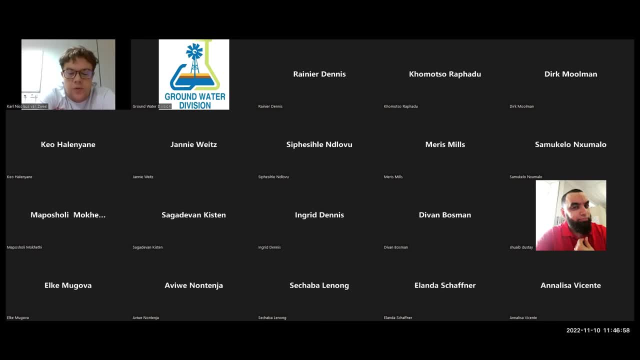 really the mean and the standard deviation, and i understand a lot of the times you'll you will have weird distributions from the data, but it's doable, so you can effectively create your own data model. so, uh, but again, this goes a bit more into the domain of multivariate statistics and uh, 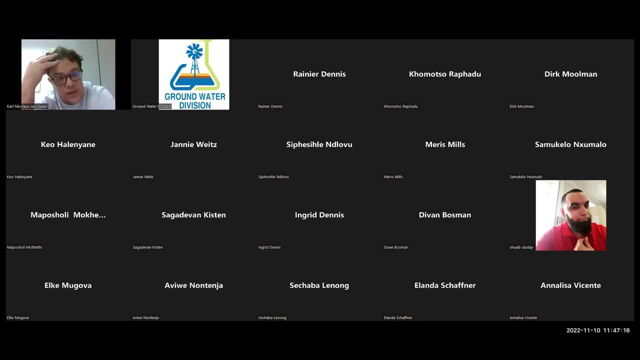 yeah, sometimes you should be a bit careful with that, but it's definitely an option, because i i did this in the beginning to just test if, uh, if it could work. you know, just a rapid prototyping to see if, uh, this type of modeling will, in fact, uh show us what we want to know. yeah, 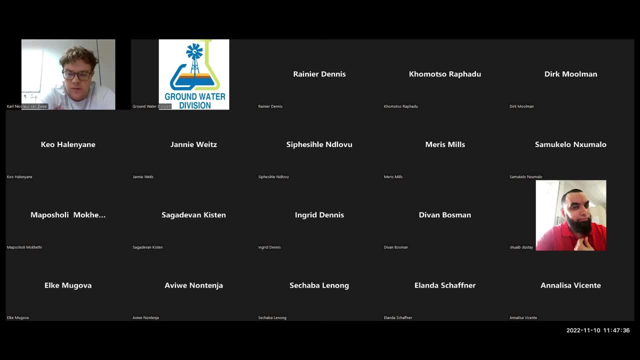 um, so i'm going to go back to the, the sampling itself. do you guys use any specialized sampling equipment? do you preserve the samples, or was it, uh, just a normal grab sample at depth and that other thing? no, um, actually, this, this, uh experimental attachment is really well instrumented, so all. 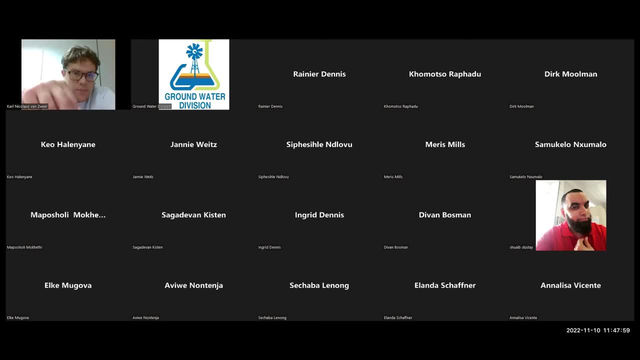 of the borals are sealed and have a um as a. it has a cup at the bottom and the obviously uh perforated uh screen and we use a peristaltic pump. uh, and then, uh, they have automatic data loggers. so in you just also. there's not a lot of water in this catchment, so uh, in in winter, for instance. a. 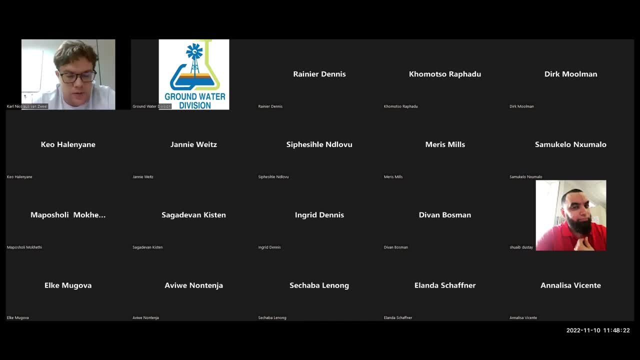 when summer a borrow might give you one liter of water in total, um, so you will pump it dry anyway, or if you pump it really slowly, you might have some uh recharge of the boral. um. so for the year, i did almost two years of my own sampling for this uh sample, so i'm going to go back to that um and 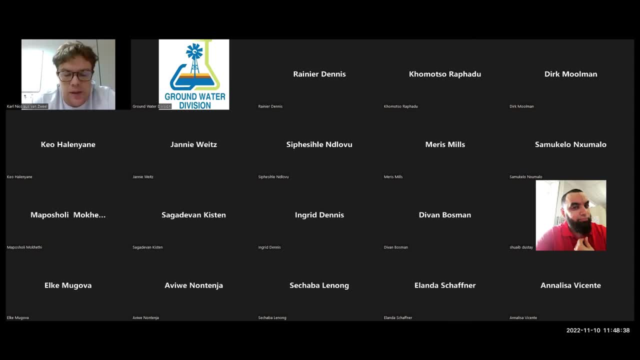 this I used a inline sampling sort of mini lab so that for probes it had a dissolved oxygen, EC, redox and pH, and so then as you sample you can measure this parameters and see when the, when they sort of stabilize, and then you can take your sample. but for the most cases, for 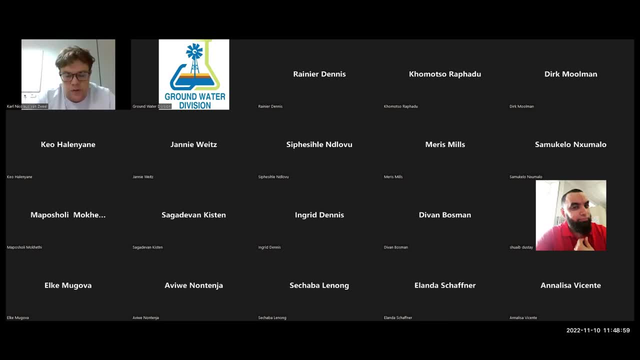 the last 10 years it was just a bit of purging the bottle until the EC stabilized, take the samples and then they come directly to the lab where we filter them in 45 micron and acidify the ICP samples and then the other samples go to the automatic sampler almost immediately. so the 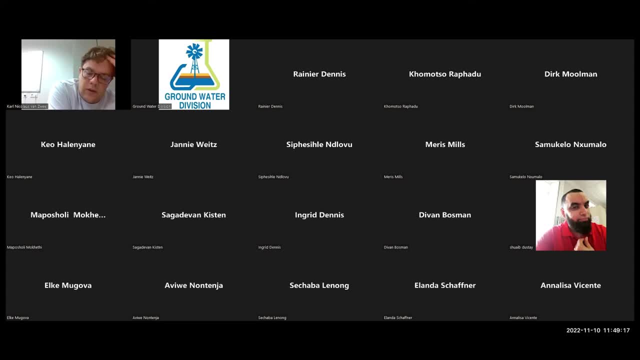 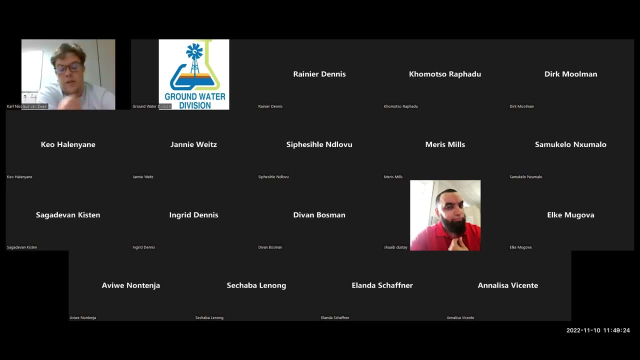 procedure in terms of the lab is really well sort of streamlined and our labs are very well equipped to handle large amounts of samples, because on average, I guess we generated about just in the year I sampled it was around 790 samples that we did. that that's quite a quite a bit. um, maybe just another question from my side. I don't see anything. 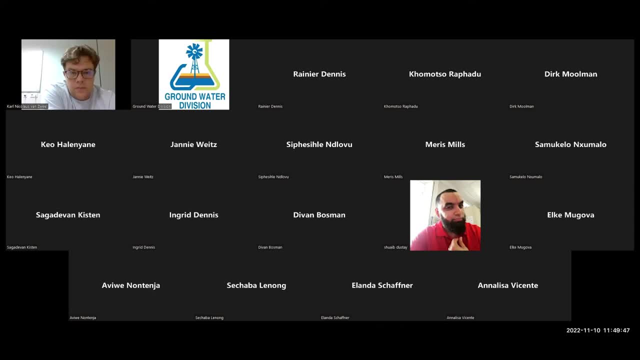 in the chat box yet, and then I'll give some opportunity for other people as well. um, so I really like your, your results, where you show the hydrograph and you can clearly see, um, the, the response of the, the clustering, as one would expect. um have you have. 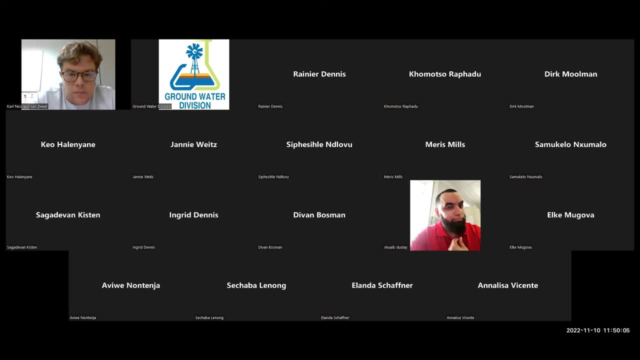 you gone to to the stage yet where you actually look at, um, uh, let's take sulfate as an example. so you're measuring sulfate at that particular flow and then what the model predicts, and and how does that compare? yeah, so this is the sort of the capstone of my PG project and what I'm busy. 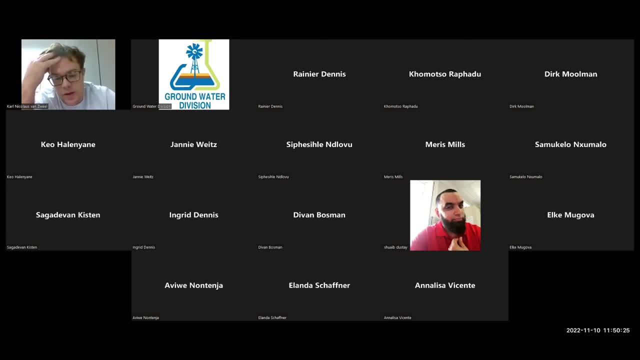 with now. we did one flood event, uh that we had 15 minutes um incremental samples so we processed about um it was a six day flood event, uh. so I don't know how many thousands of samples there were, but obviously we didn't analyze each sample. we looked on the hydrograph and just sort of selected. 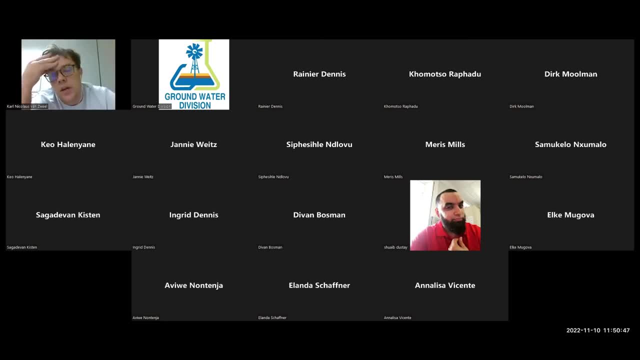 um, in areas where you have to change in concentration, and for this we have major cations, anions and stable isotopes. so this is now. the last part is to to. so we'll do hydrograph separation with stable isotopes and then compared to what my model is doing to see. 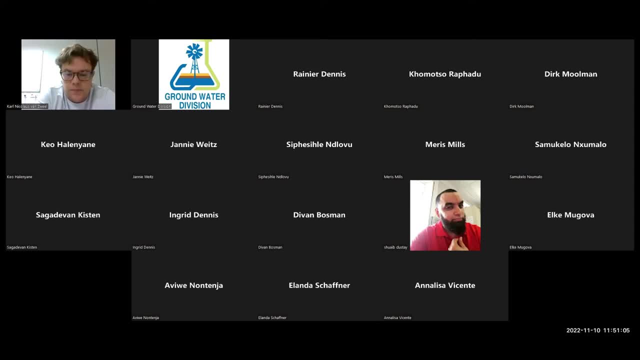 how effective it is. any any questions from from from the floor for Niklas. um, I've got one year. uh, given the importance of alkalinity in your modeling, how confident are you that the results, particularly for groundwater, are representative of subsurface conditions? so you have to understand in the 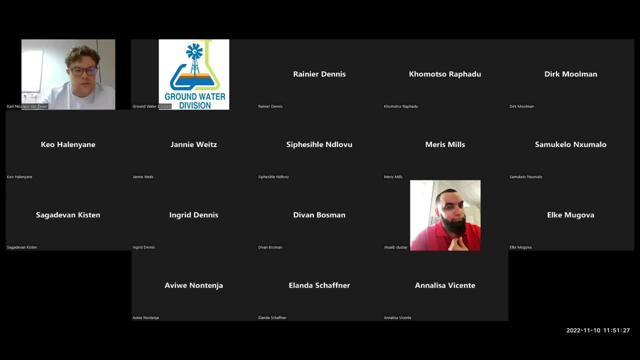 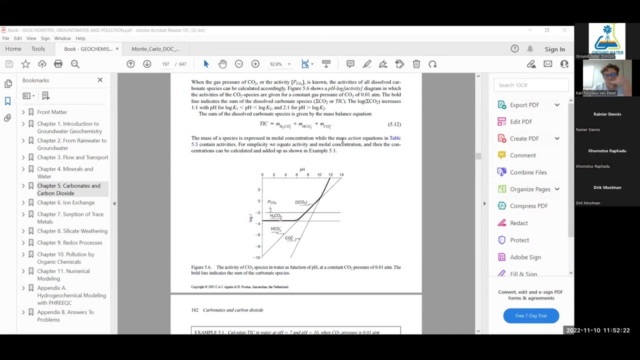 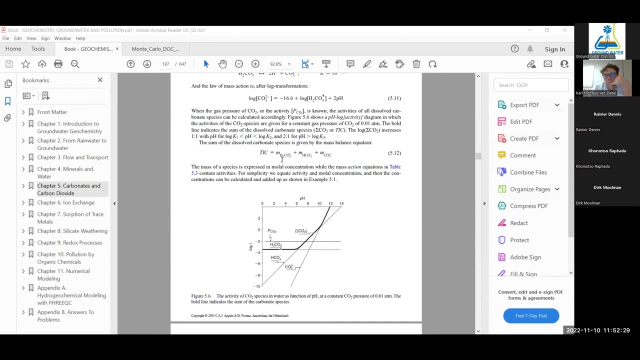 carbonic systems what alkalinity is. I can maybe just show you. so trc is total inorganic carbon, right, but this is in fact um what you're measuring when you, when you're measuring total alkalinity. so you, what total alkalinity is is a is a combination of various carbon species, but some 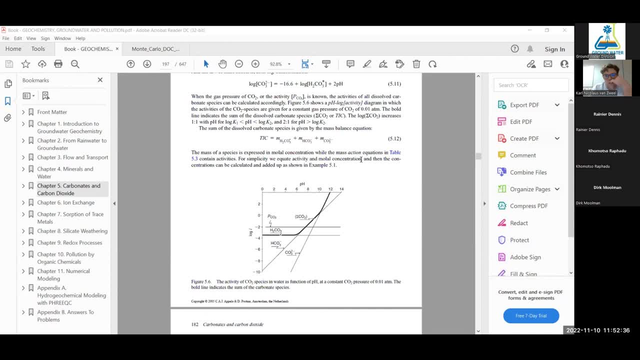 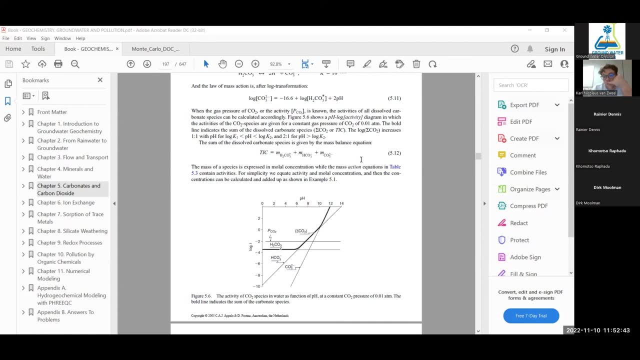 of them do not exist in certain pH ranges. so if, for, in fact, you, in most cases in in aquifer systems, you measure total alkalinity and you have the pH, you can define the, the concentrations of your other species. so in our case, we actually modeled uh, we actually measured total alkalinity and we measured uh pH. 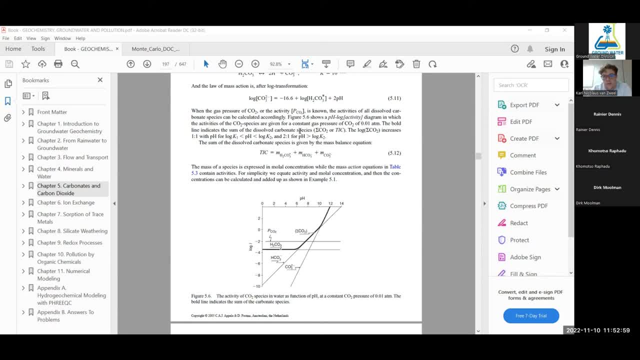 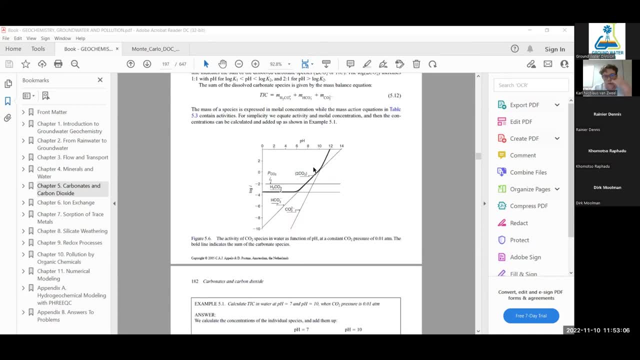 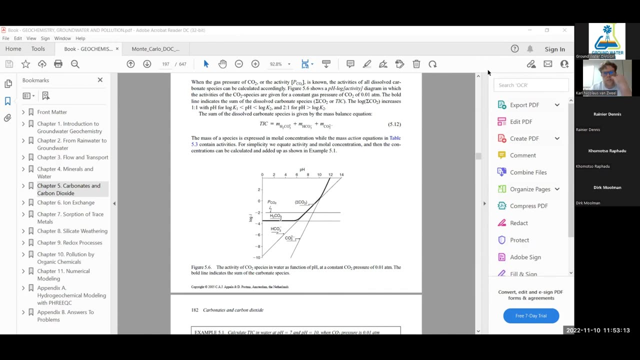 both in situ and in the lab. so we're fairly confident that we could define all the other species in terms of um, of using them, the relation of what uh, what uh, you know what the total uh or what total alkalinity is. I don't know if that answers your question completely. 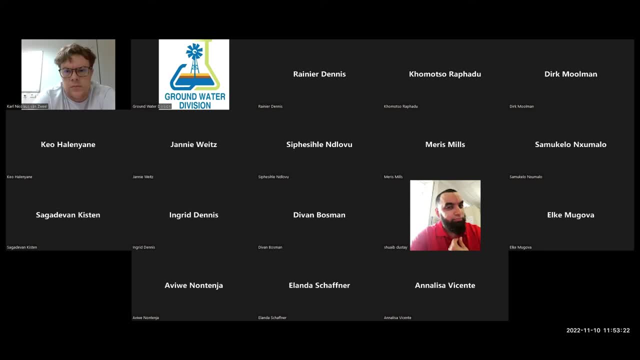 yes, any, any any more questions from from the floor? yeah, well, if you guys think of something you you're welcome to to post in the chat and, um, if uh, after our our webinar, if there's some more questions, we can always uh get them to to to. 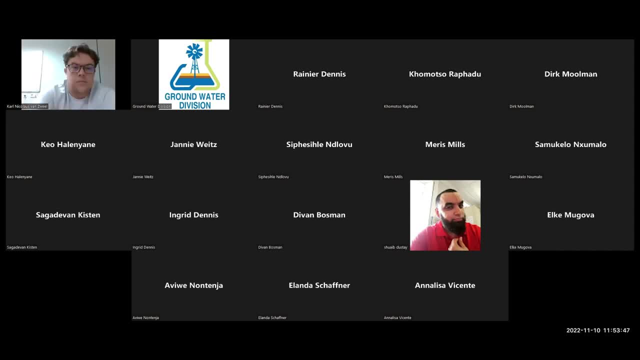 Nicholas to answer. um, Nicholas, we, we want to thank you for the time. I'm looking at at 10 o'clock here, we're almost going for our low cheating, something that you guys in Europe are not used to- and uh, so we, we plan our days around that and um, yes, we, we wish you all the the best of luck. 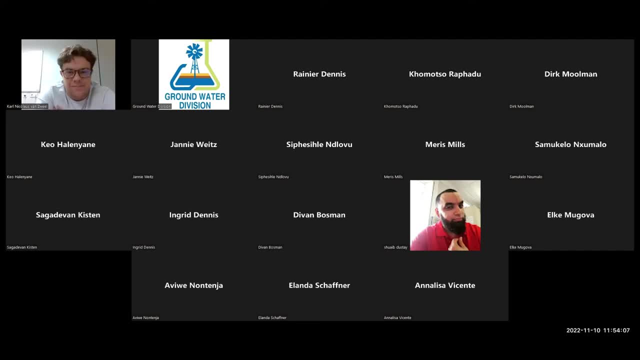 uh, completing your, your PhD and then, um, yards of heard a little birdie sing. it seems like you're not coming back to South Africa, looking at other opportunities abroad, and that's actually a shame to tease in South Africa, but nevertheless, um, it's always be home for you and and uh, the best of luck.